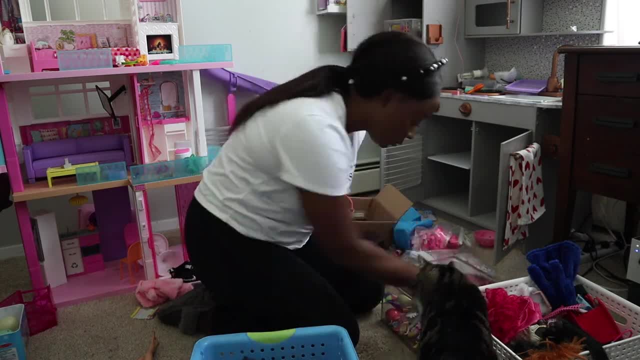 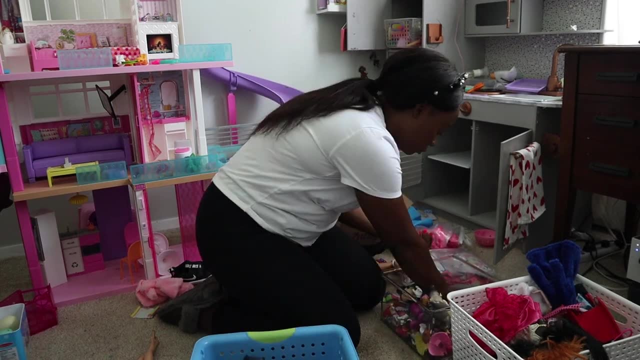 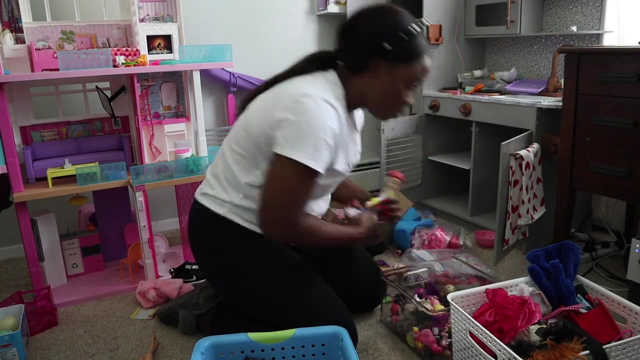 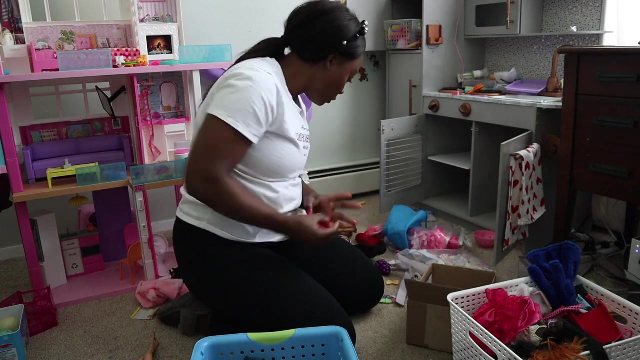 If you guys have kids, then you know how easy it is for toys to literally take over the space. So today I'm gonna be tackling our playroom and decluttering, organizing and cleaning all of Riley's toys. I'm starting off by just going through all of her figurines. 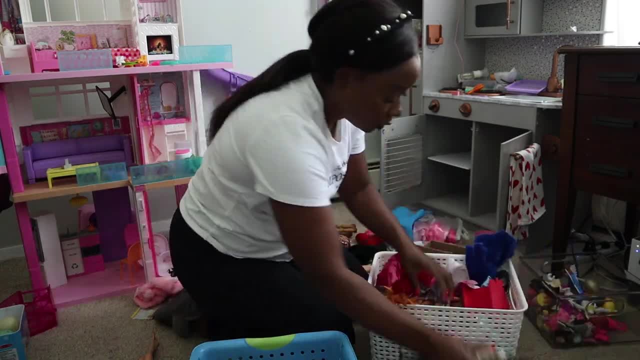 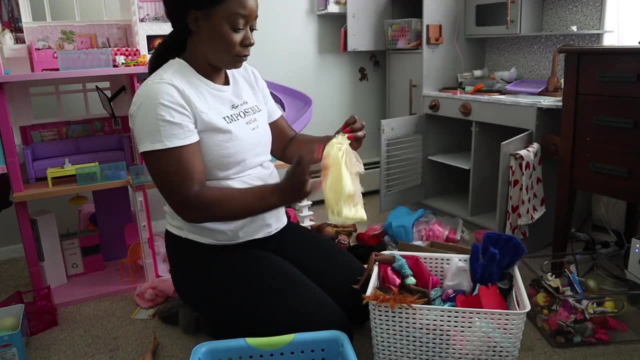 and I started with a basket, and this basket is a little bit of a mix of things I wanna throw out and also things that I'm going to donate. Little bit later on in the video I will then start to separate and have a bag that I'm going to be throwing away. 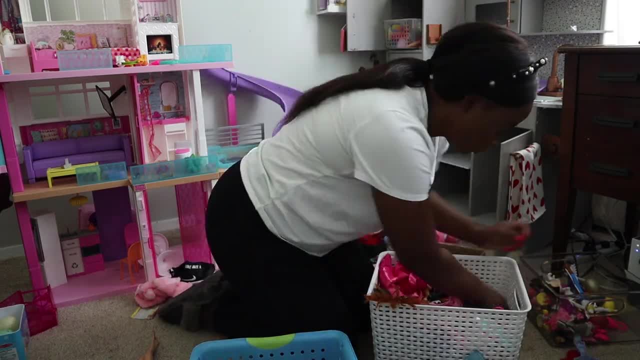 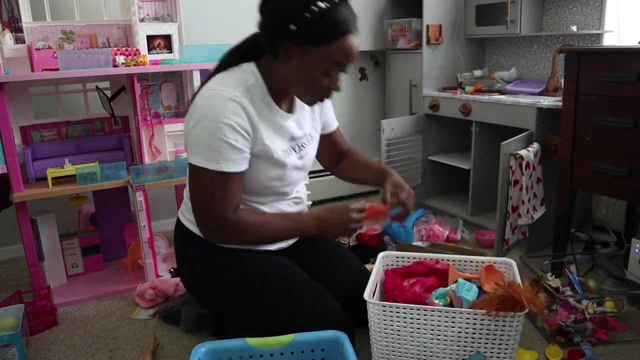 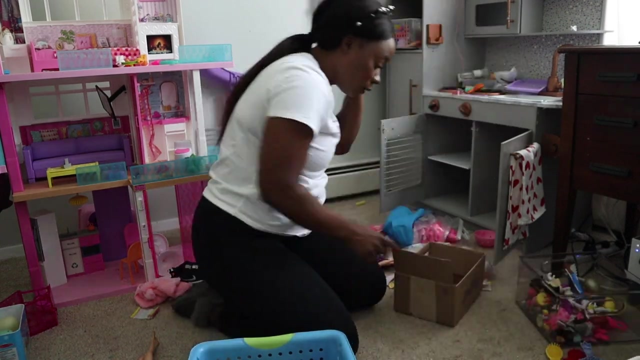 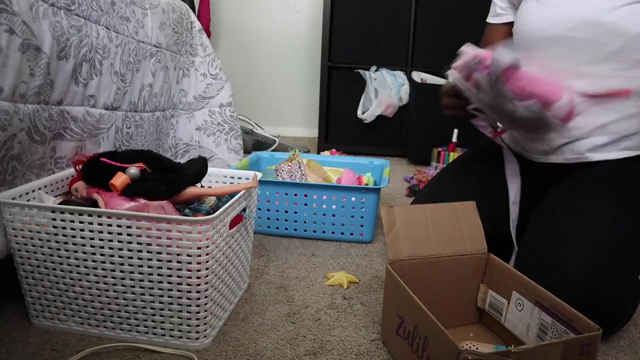 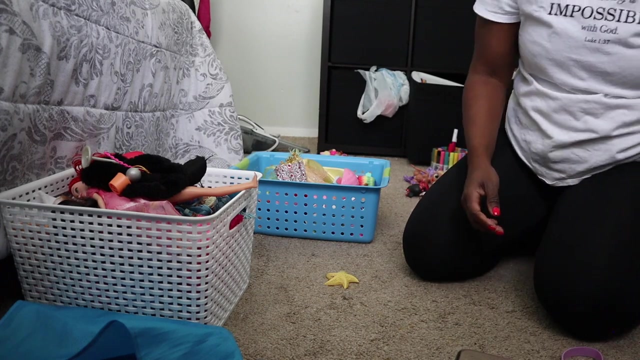 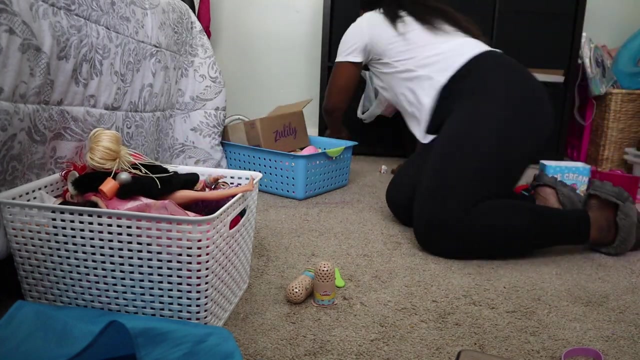 and then also a smaller bag of things that I'm going to be donating. This is basically my family. I'm putting these in the 사막 and then these are the things I'm gonna be using them for. I'm gonna be using the bigger one. 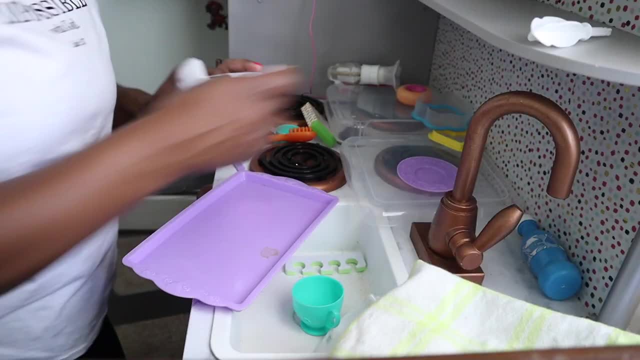 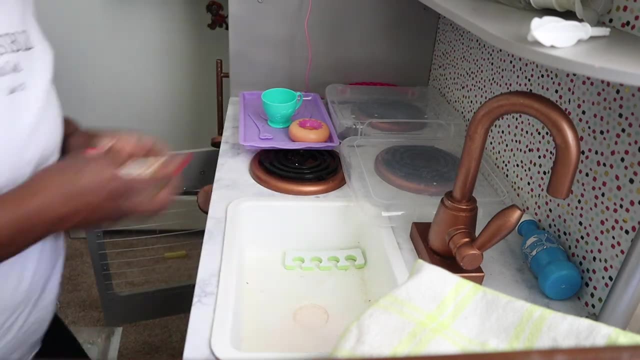 and this one's gonna be for the smaller one. I'm gonna be using this as a blanket, because we have a lot of things that we're gonna be doing and I'm gonna be putting these together. So there you have it, the small bag toys. 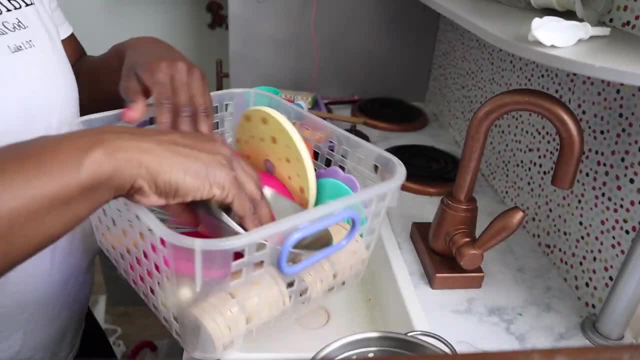 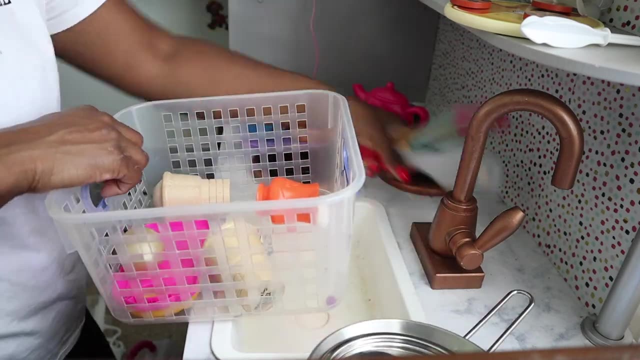 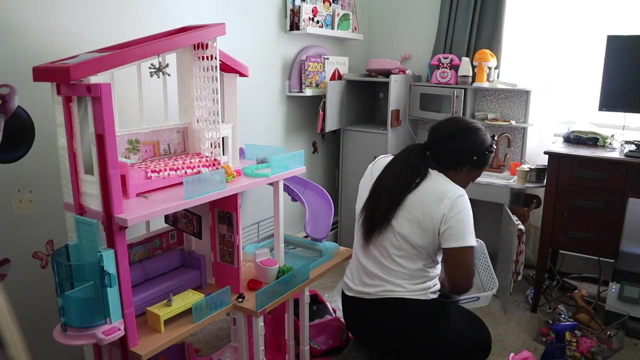 any time I'm going through Riley's things- whether it's toys, her clothes or anything like that- I always hesitate on which items I should donate or throw away, because typically what ends up happening is, as soon as I get rid of them, she starts to ask questions as to where this particular item is, and I 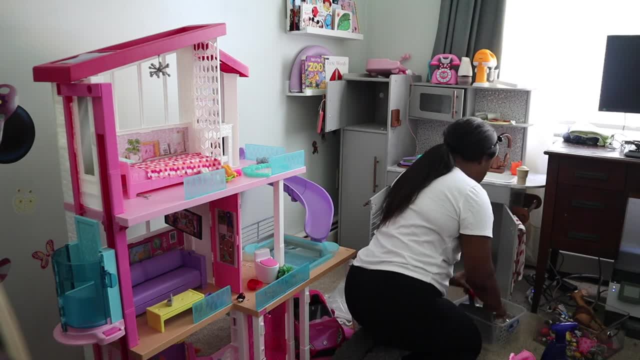 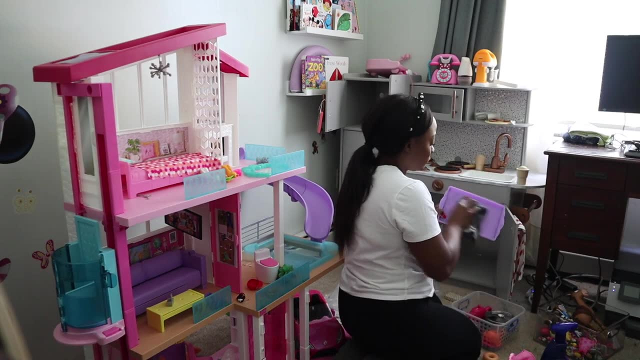 literally just have to play stupid and say, hey, I have no idea what happened to it. sometimes I like to hold on to things just a little bit longer to see if she sparks any interest in them. let me know if you guys experience the same thing with your kids. 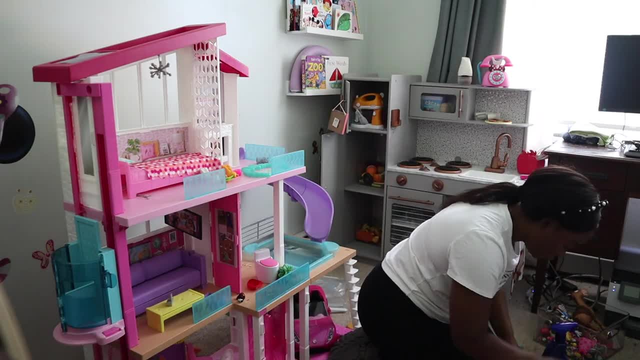 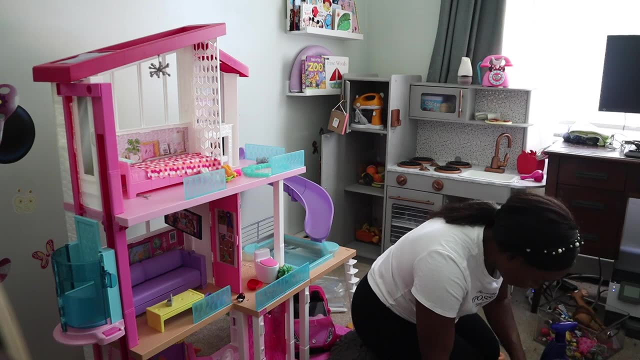 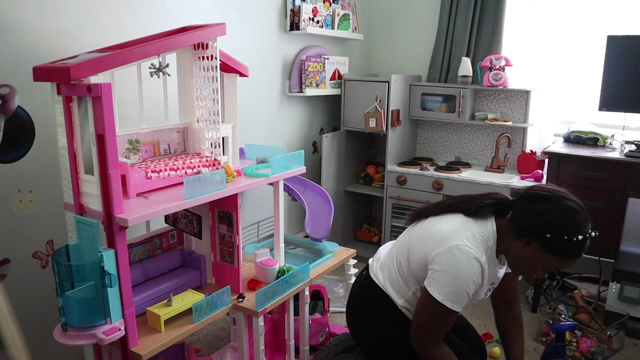 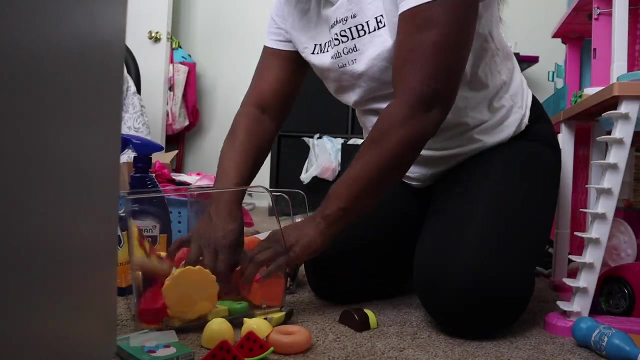 tell me how to be closer to you. tell me how I'll do it, babe, cuz I just wanna make you feel what do about you? just tell me how to do it, babe. I love it when you whisper in my ear. words only meant for me to hear. 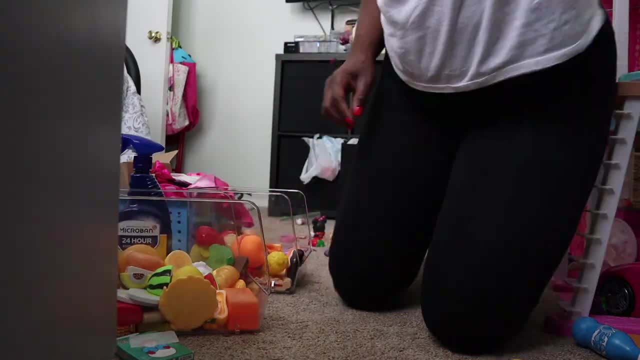 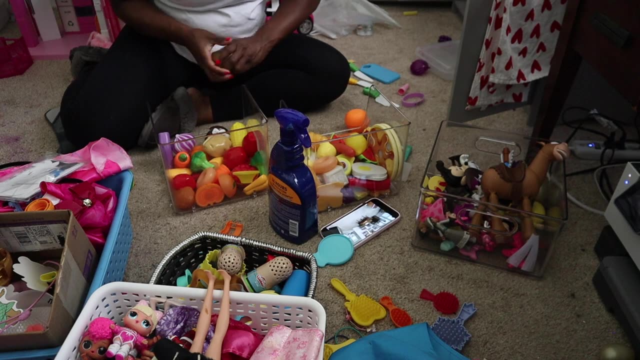 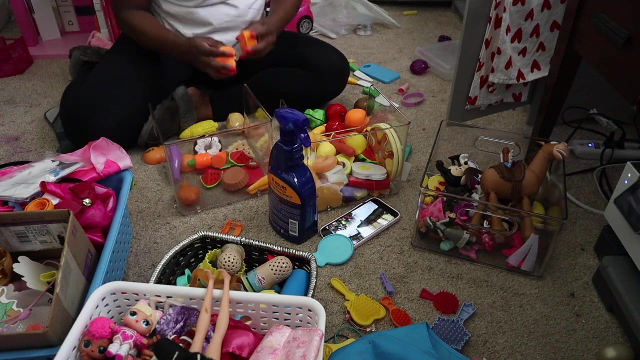 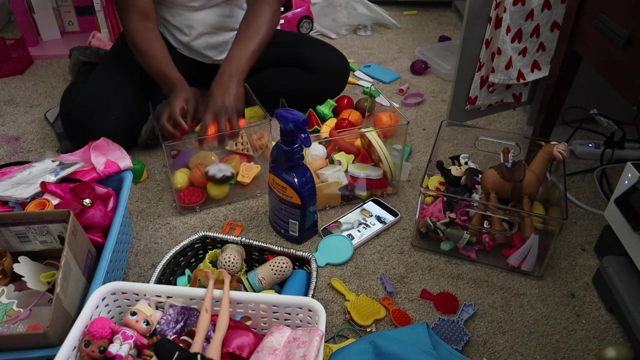 promise that your secret's safe with me. You're the only reason. yes, you're the only reason. Baby, you're the answer to my prayers, Feeling like the world is in our hands. Now I know what this is meant to be. You're the only reason. yes, you're the only reason I'm free. 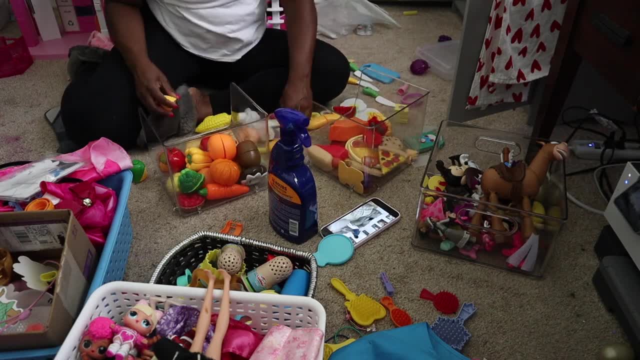 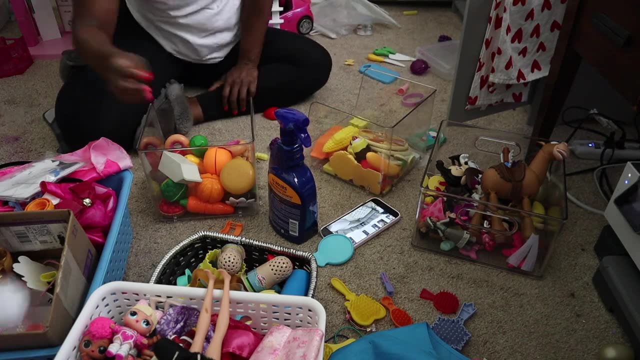 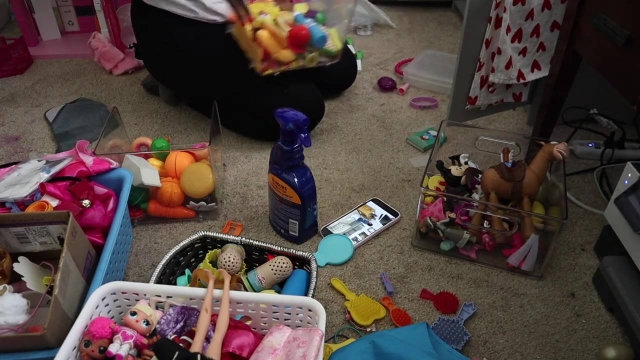 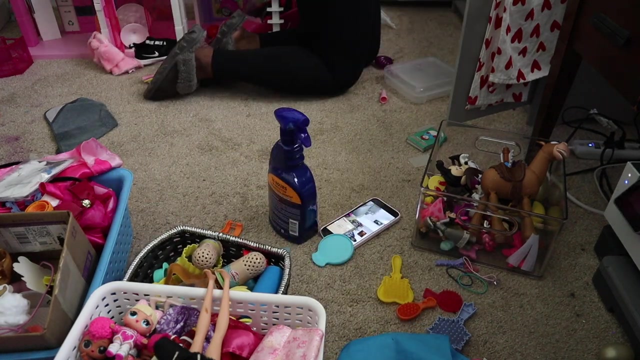 You and I could run away now. You and I could be on a raid, But I come back for some sweet, dried change Of aversions. No time to waste. You're the only reason- yes, you're the only reason- I'm free. You and I could run away now. 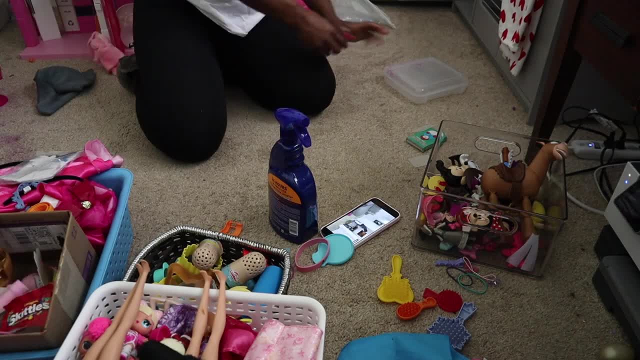 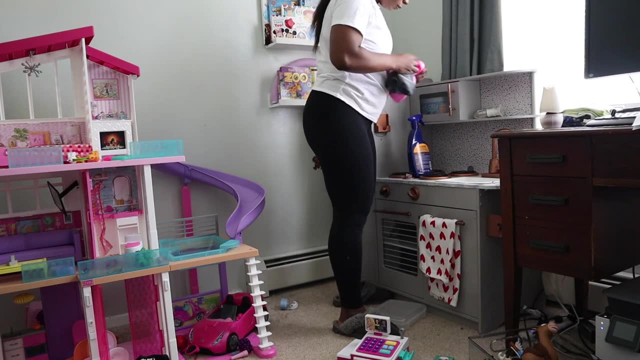 to wipe down her play kitchen. I'm going in with a microband 24-hour multi-purpose cleaner in the citrus scent. to be honest, I don't smell a citrusy scent at all, but it does say that for 24 hours it's gonna keep killing 99.9% of bacteria, also with 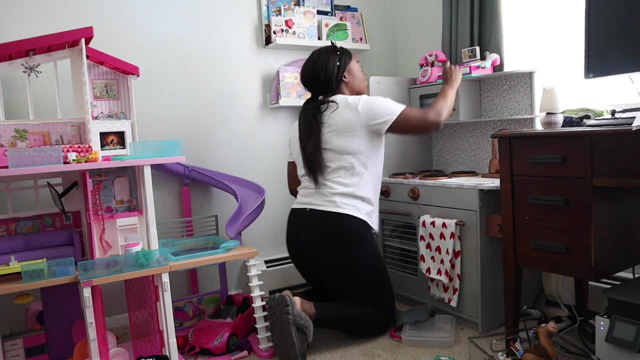 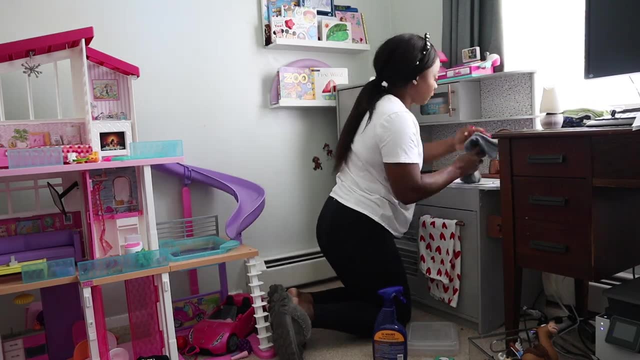 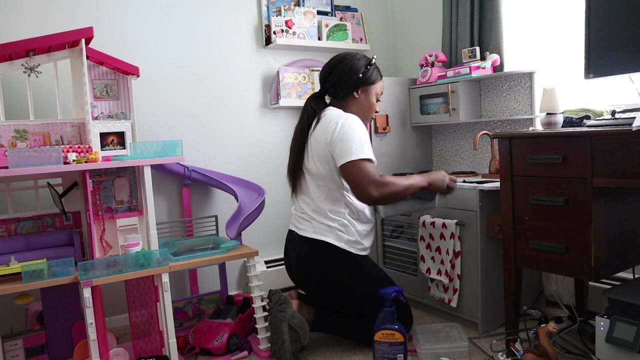 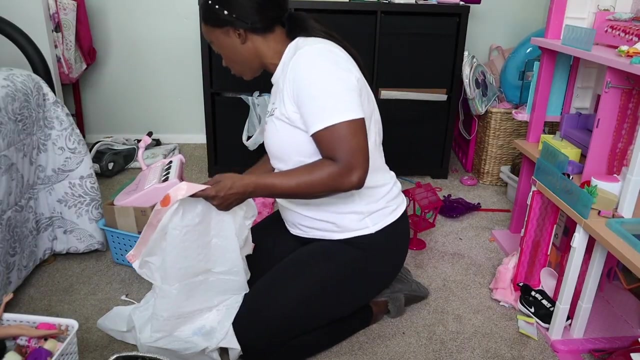 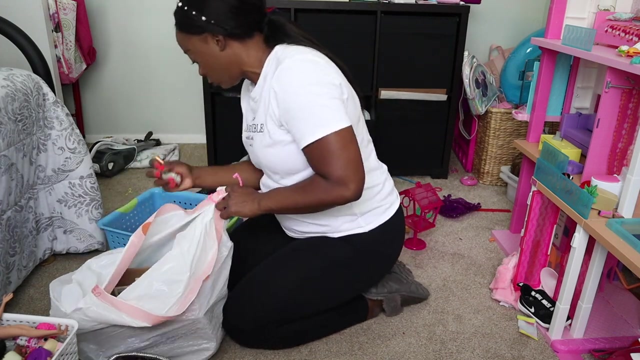 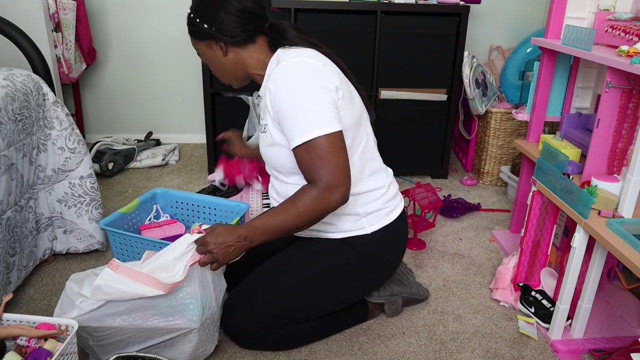 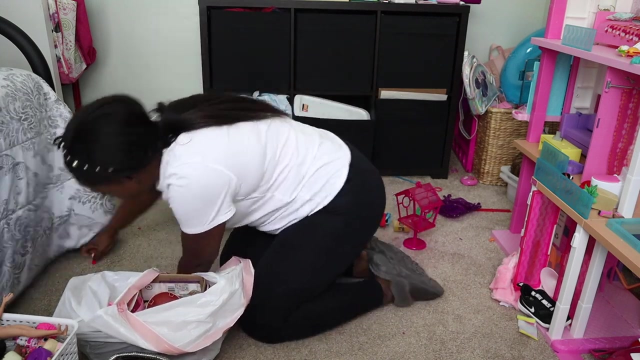 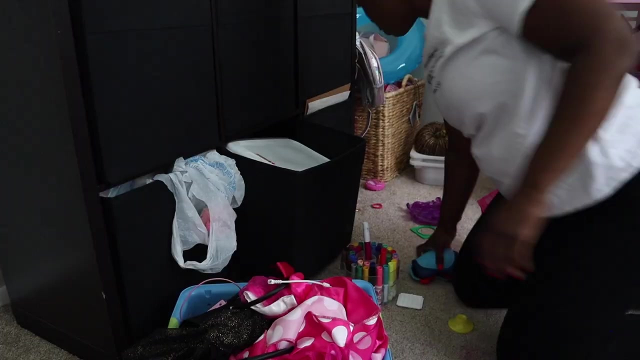 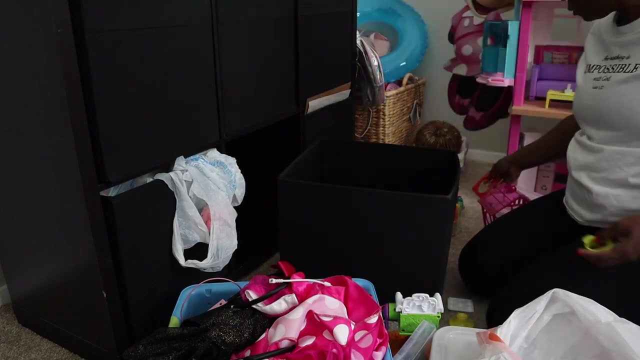 the cold that's been passing around. I definitely want to make sure that we are tackling any germs or anything like that to help reduce the spread of any type of sickness. so, as of right now, we have been using the bins to store different books and crafts and all of that kind of stuff. 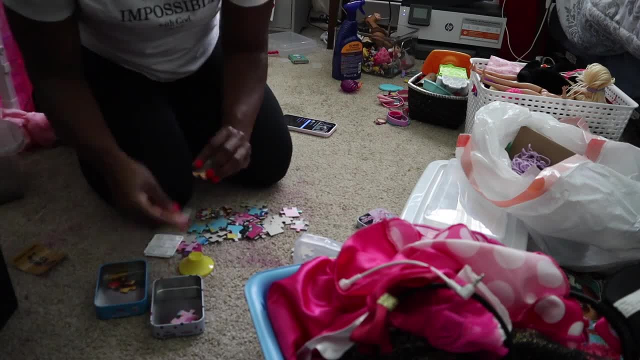 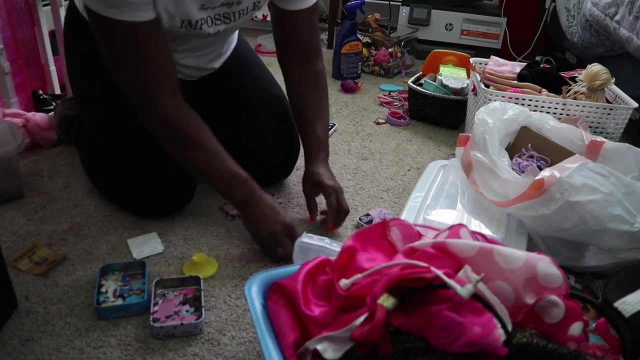 and I'm finding out it just is not really working for us at the moment. so what I ended up doing is I ended up bringing the craft cart that I had upstairs in her bedroom and I decided to bring that downstairs and organize all of her crafts, puzzles and all of that stuff. so you guys will see that a little. 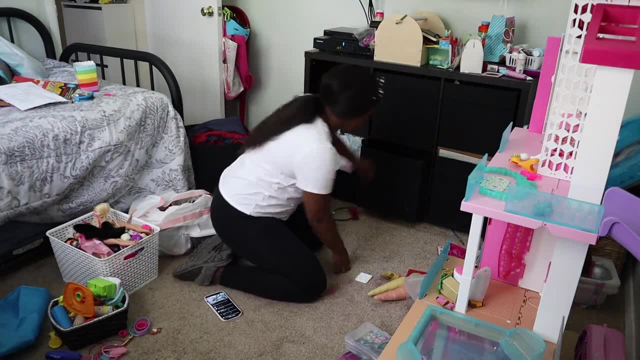 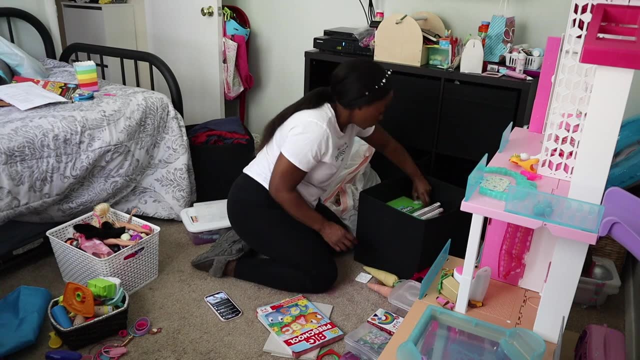 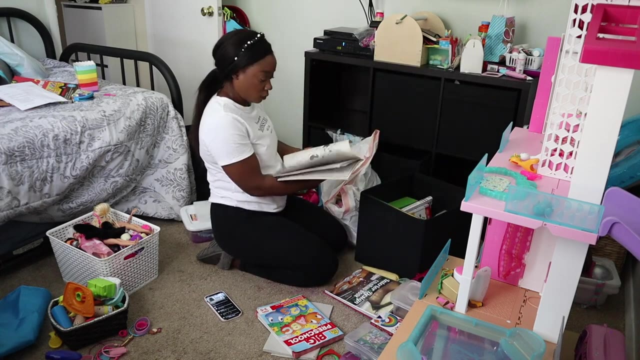 bit later on in the video, I think it's just going to work for us a little bit better. but that is the thing. when it comes to organizing, you have to literally just play around with different things and see what works best for your lifestyle. crashes gone, we doing it wrong, baby you and baby you and I just start living. 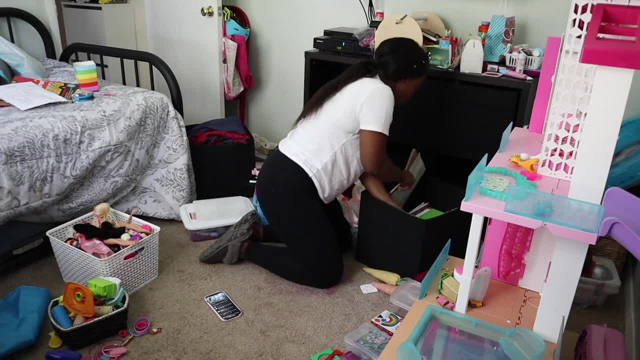 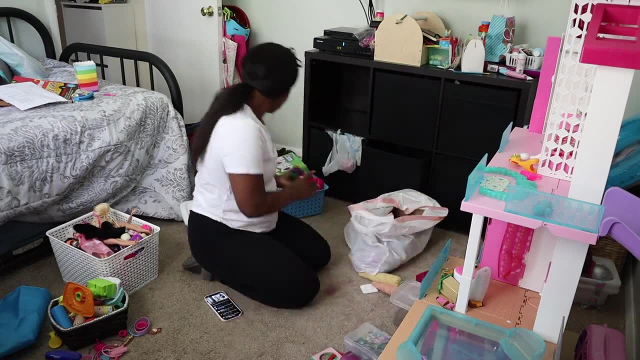 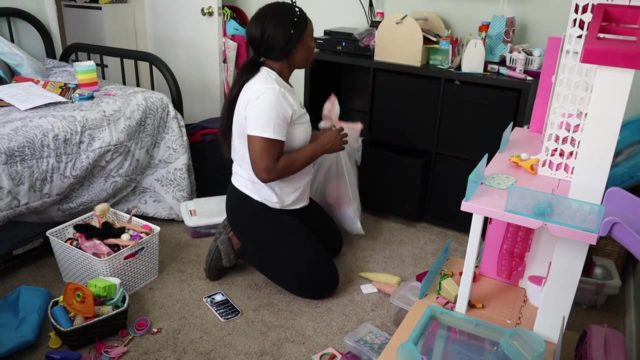 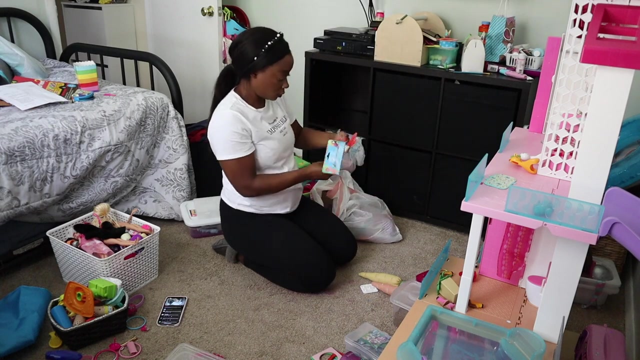 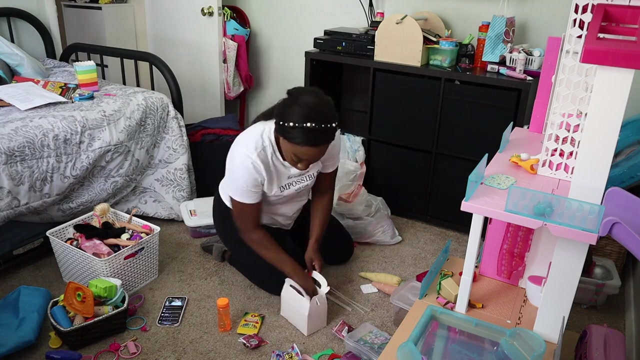 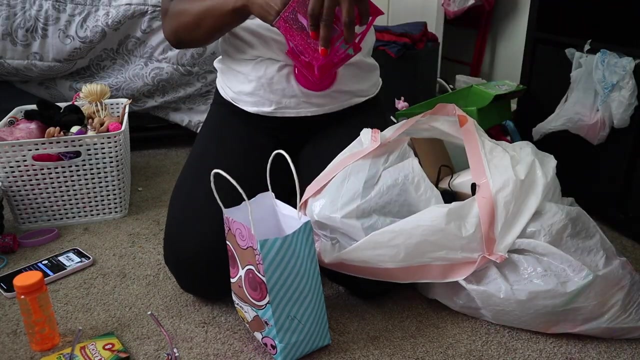 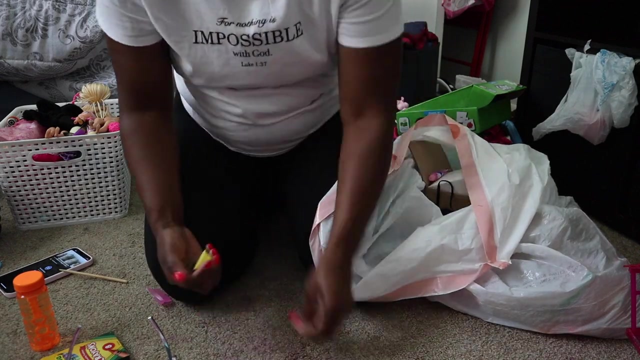 now the whole high we. there was nothing, baby we own. Oh, I don't wanna cry, I don't wanna waste my time. So, baby, we should start living now. Baby, we should start living now. We are close. can you feel it? Something is behind the clouds. 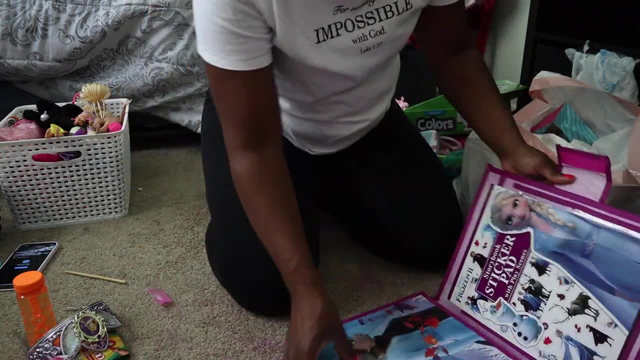 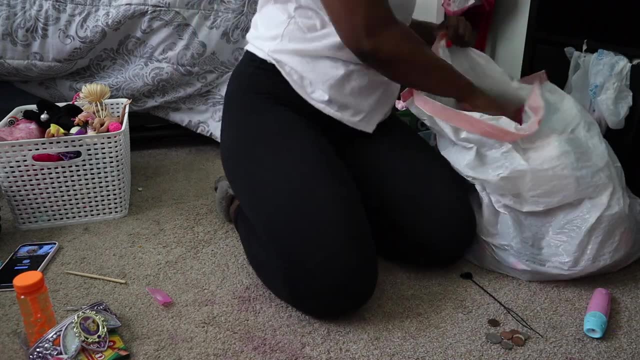 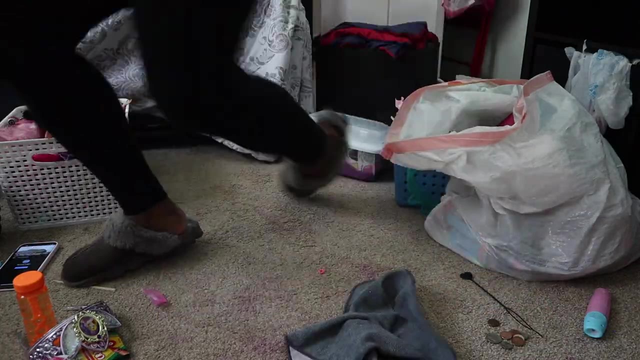 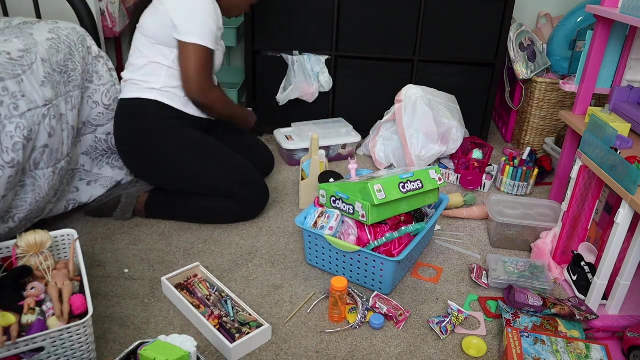 We just have to believe it That we can make the sun come out. Let us lose ourselves in a fairy tale. Who can say what's wrong or right? We're the only ones who can decide, Baby, you and I. As you can see, I brought the cart down and it fits perfectly in this corner. 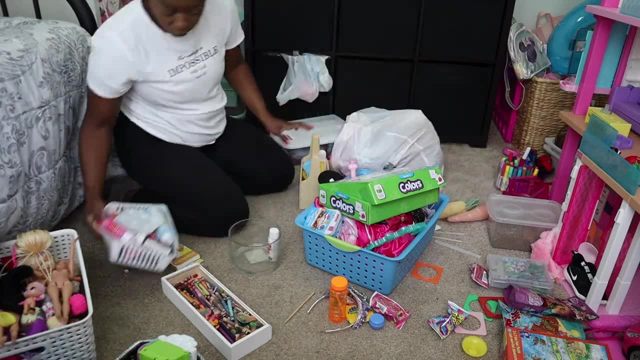 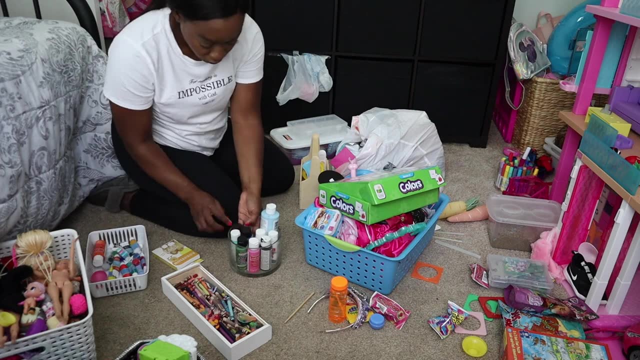 And now I'm going to show you how to make a cart. I'm going to start taking anything that was at the top of the black organizational furniture piece And I'm going to try and organize it as best as possible so I can put it on the cart. 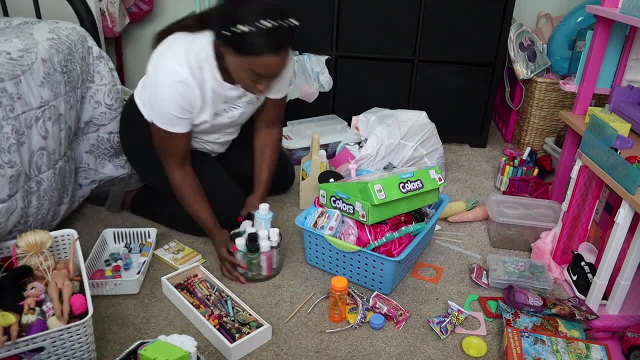 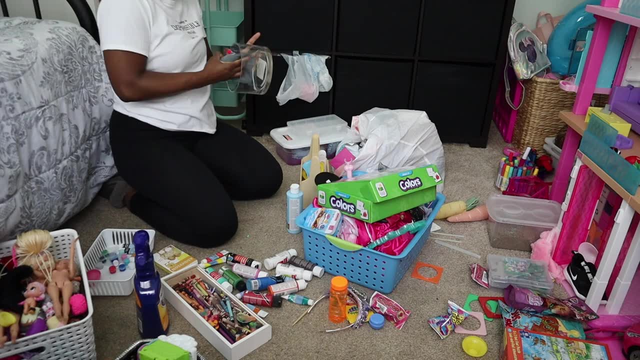 So we had this old dish for the longest And I was actually going to throw it away And I thought what better way than to store all of her paints and all of that stuff And everything fit perfectly. So I'm going to put everything in here. put that at the top of the cart. 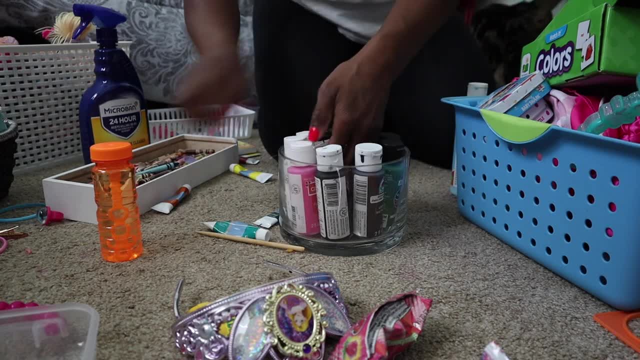 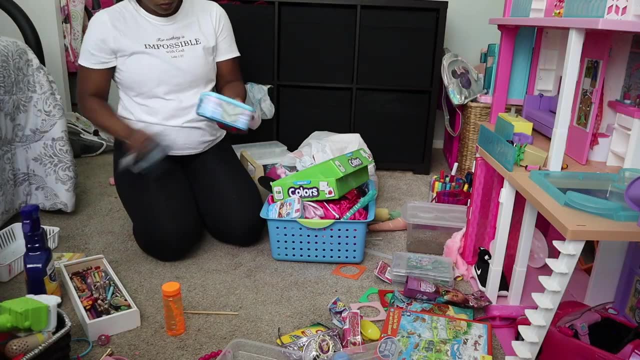 And then I'm also going to remove all of her crayons From the cart, That other wooden piece, And I ended up using this container that her perfume came in, That I had shown you guys in a previous video that our neighbors had gotten her. They fit perfectly as well. 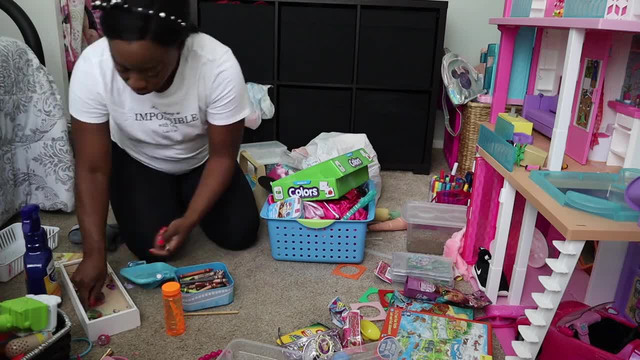 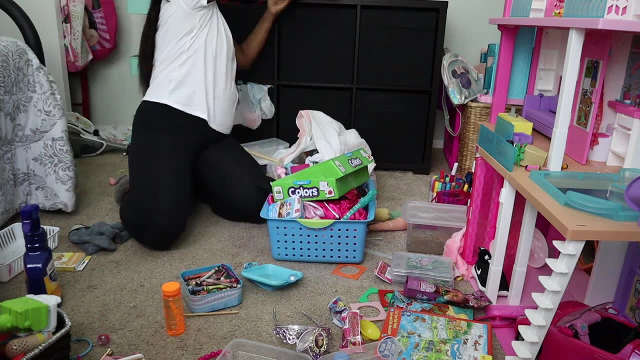 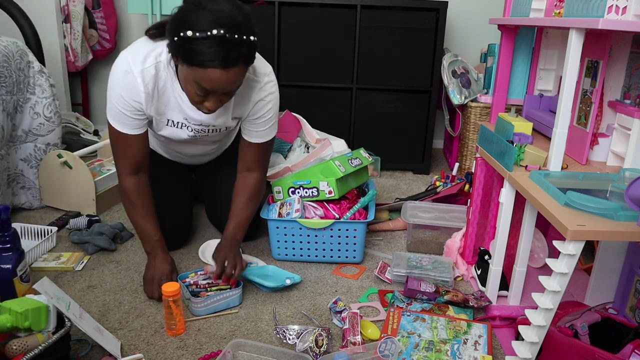 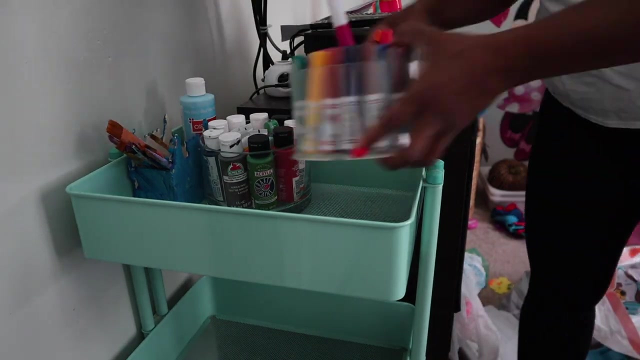 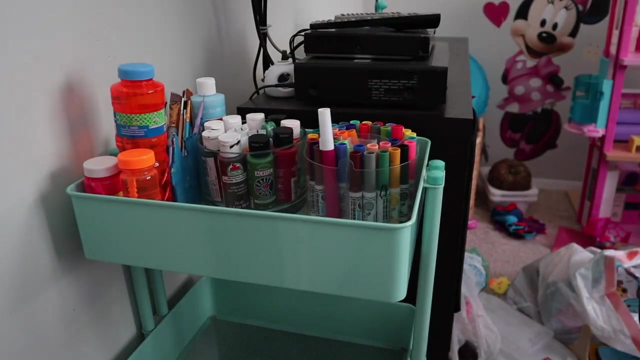 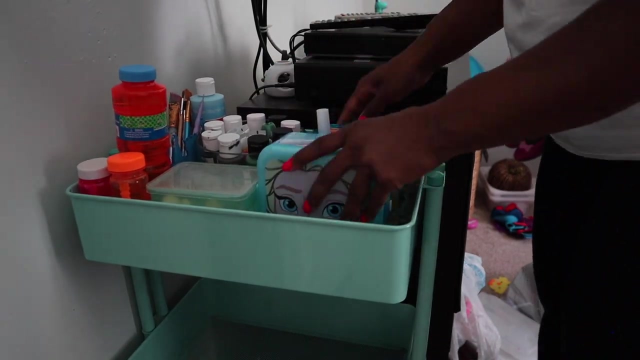 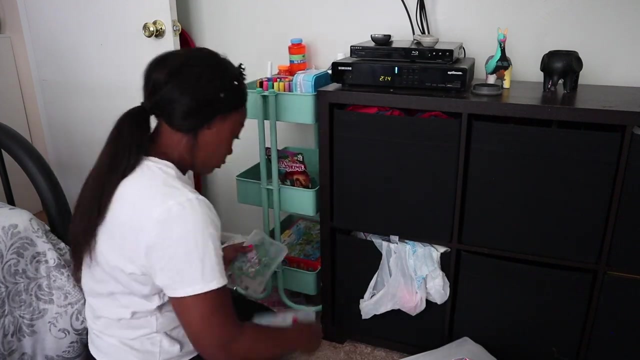 And it's just a nice way to organize all of that stuff. So that is basically what I'm doing. I'm just trying to repurpose the things that I already have So to make a better use for the space In here. we add in the Manaze: 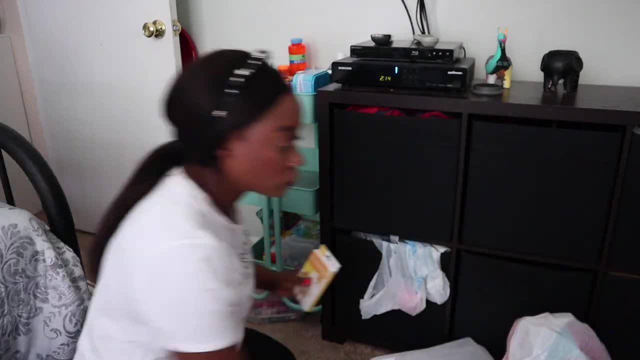 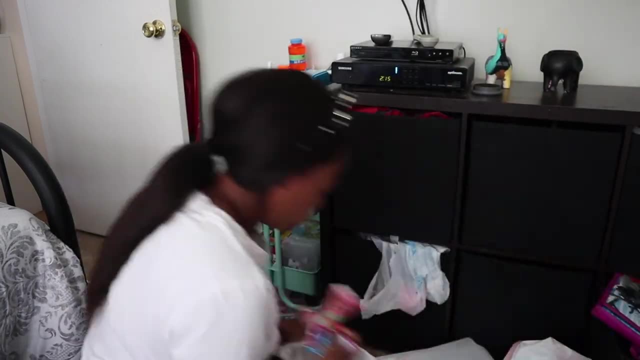 Then this is where I'm going to put my printer, And the one thing you have to notice is that you just don't want it for depth. I made the border here to match the completely wide side of the tower. I'm thinking you were made for me. 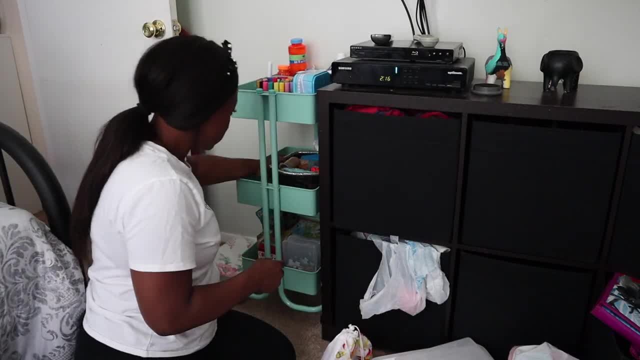 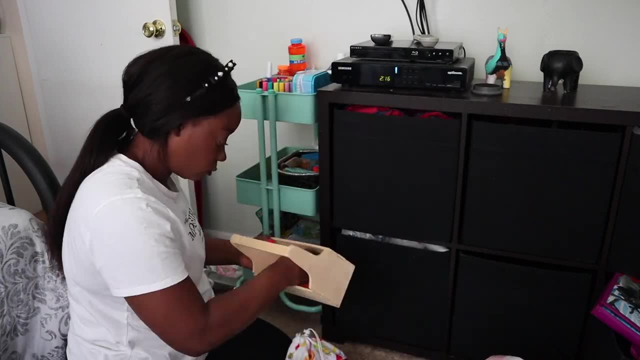 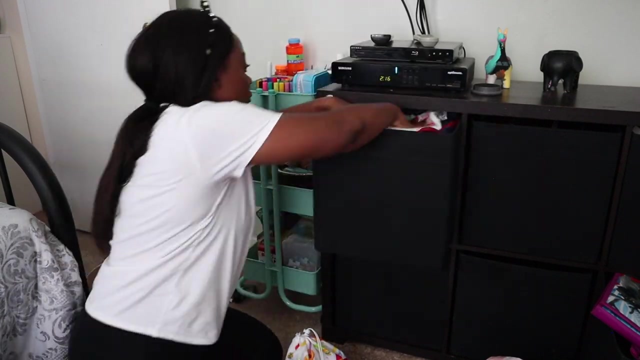 Isn't it my birthday yet? Cause I gotta say You're looking like a gift for me, Wrapped up, nice and neat. baby, Get in my way now, don't be shy. We'll be here dancing day and night. Get in my groove now, don't be shy. 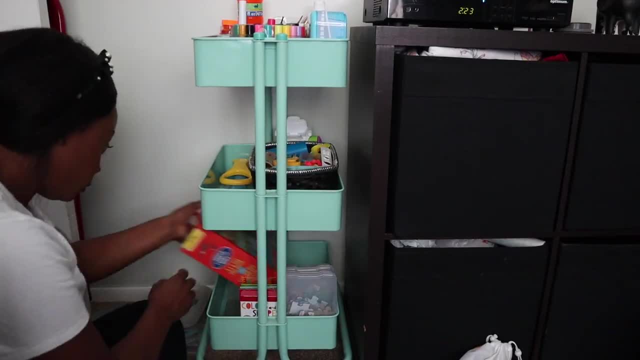 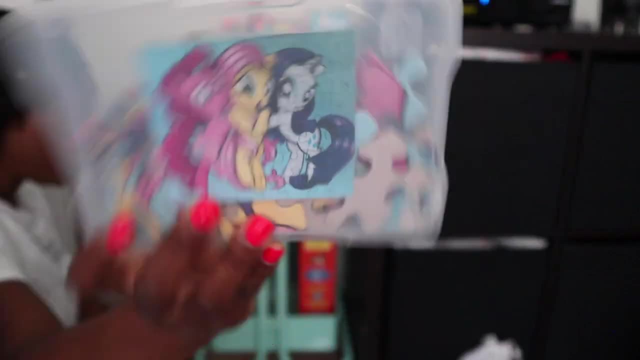 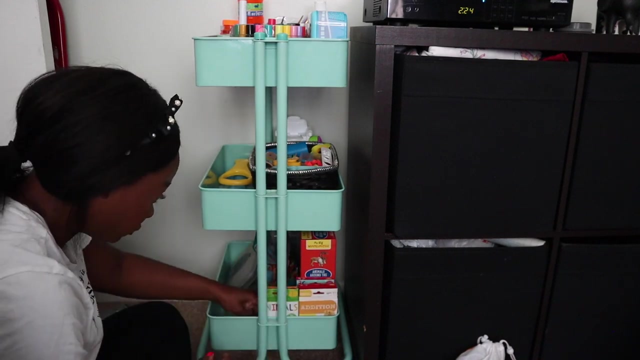 Cause I got this system of favorite things. It can definitely be hard trying to organize and keep all of the puzzle pieces together, so a really great hack that I've been using for years now is picking up picture cases. I got these from the container store and I like to store all of her puzzle pieces in there. 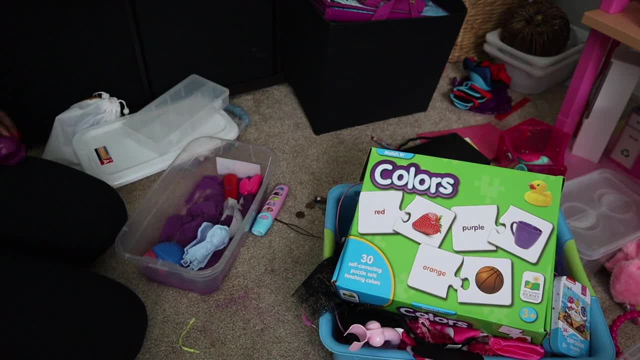 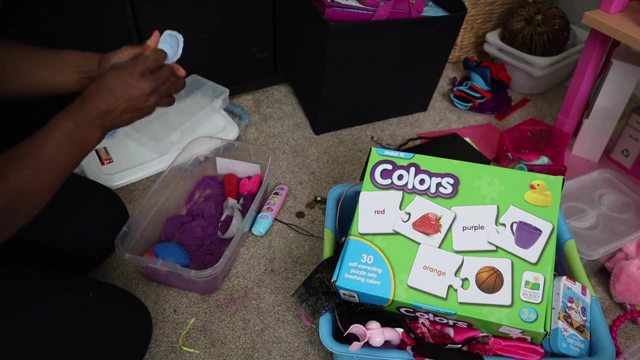 Also. what I like to do is I will take a picture of the puzzle already finished. I will take a picture of it on my phone, print it out on the printer, cut it out and then tape it to the front of the case. 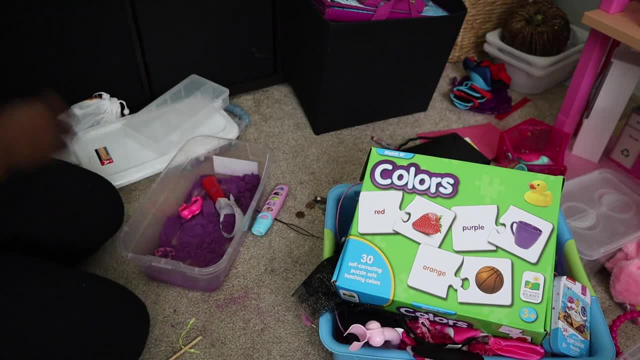 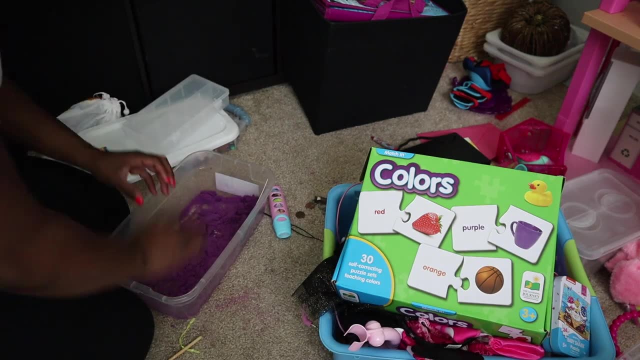 This way, you know which exact puzzle it is, so it just makes it easier when you're trying to find a fun puzzle to do. I will show you how you can catch my vibe, And right away. I got so much time Looping in the blurry lights. 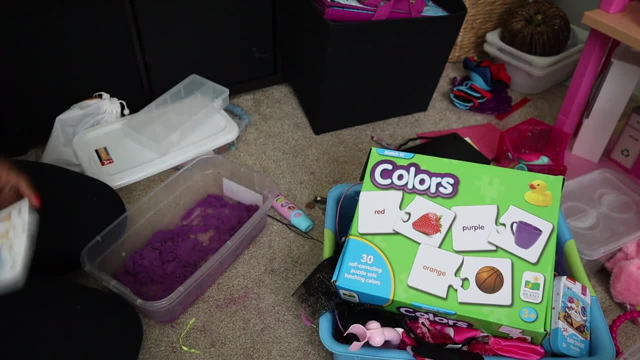 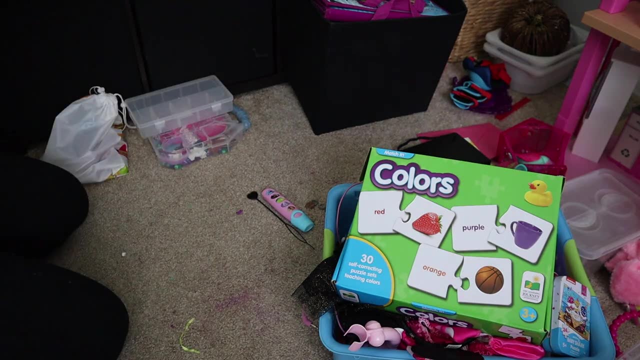 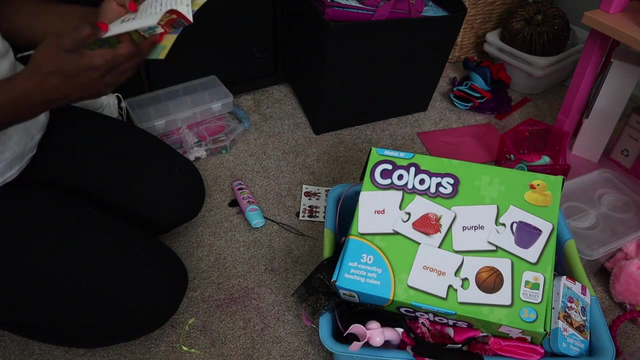 Get in my way now, don't be shy. We'll be here dancing day and night. Get in my groove now, don't be shy, Cause I got this system of favorite things. You could be the part where it all begins. You could be the first and the second. 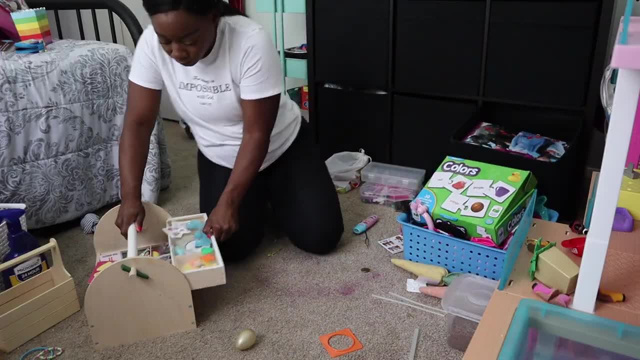 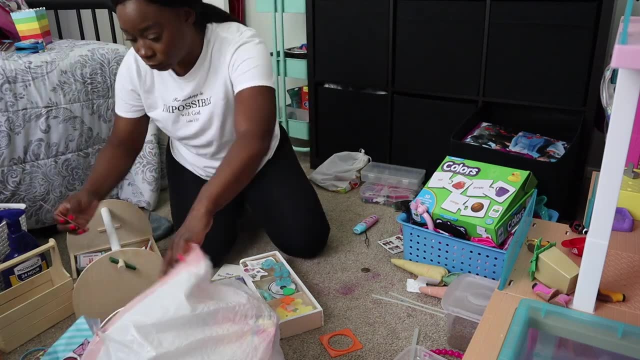 and the third and the rest of it. You could be one of the things I long. Sunday morning breakfast with my bedroom door locked, I like every deal and there's a cherry on top. Get on my list of the things I love, love, love. You could be the one I trust. 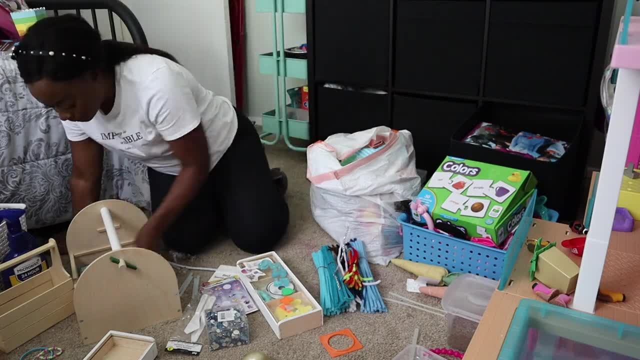 For the second chance to say, oh, nothing for us. I like it how I put the cherry on top. Be one and trust. love, love, love. Get in theround with the cherry on top. Get on my list of the things I love. love, love. 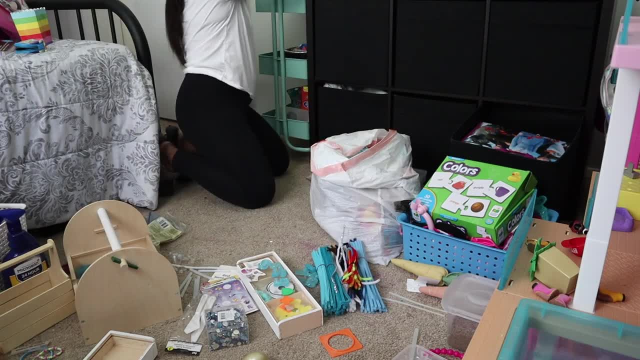 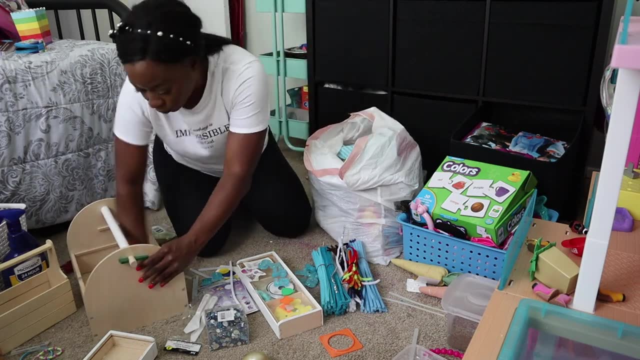 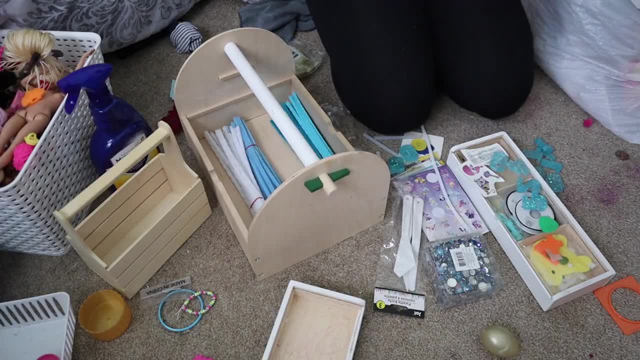 The things I love, the things I love, The things I love, love, love, love, love The things I love, love, love, love, love The things I love, the things I love- Cause I got this list of my favorite things. 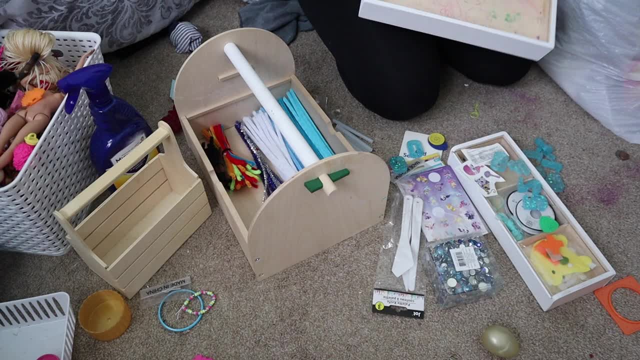 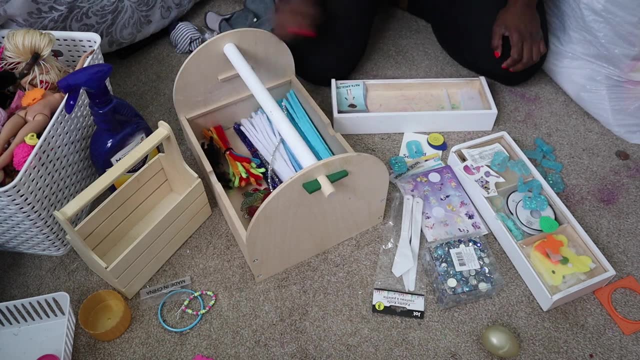 Cause I got this list of my favorite things. Cause I got this list of my favorite things, You could be the part where it all begins. You could be the first and the second And the third and the rest of it. Get in my way now. don't be shy. 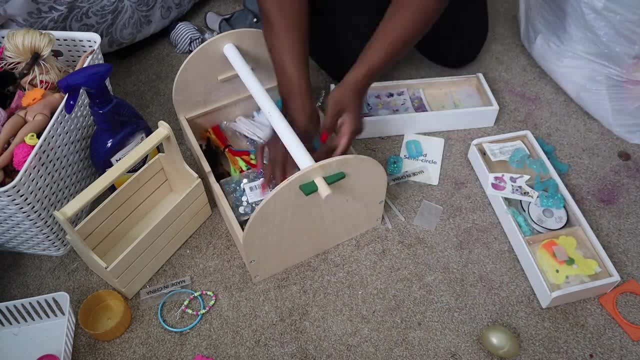 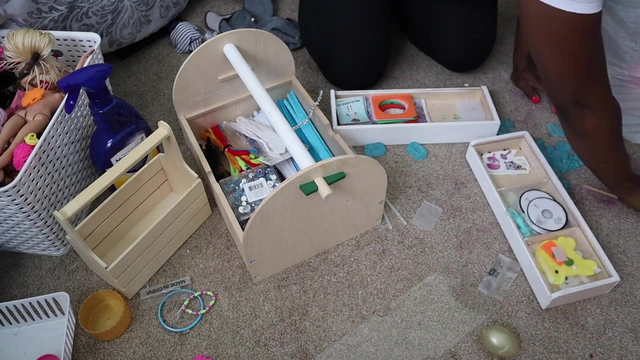 And we'll be here dancing day and night. And we'll be here dancing day and night. Get in my groove now, don't be shy. Get in my groove now, don't be shy. You could be one of the things I love: Sunday morning breakfast with a bedroom door locked. 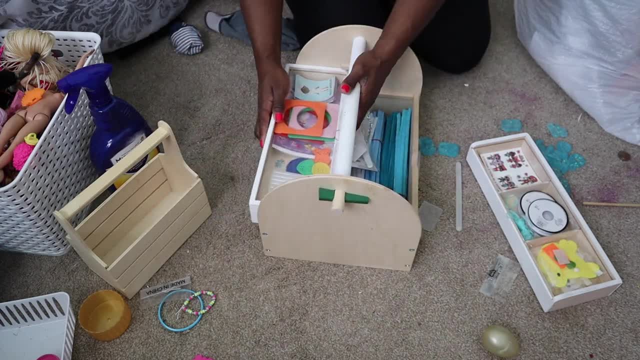 Yeah, like every tingling there's a cherry on top. Yeah, like every tingling there's a cherry on top. Get on my list of the things I love, love, love. Get on my list of the things I love, love, love. You could be the one I trust. 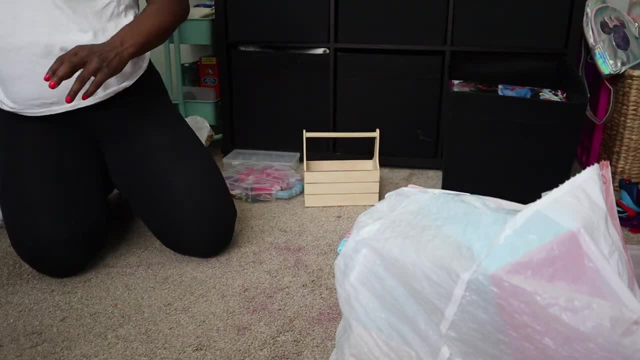 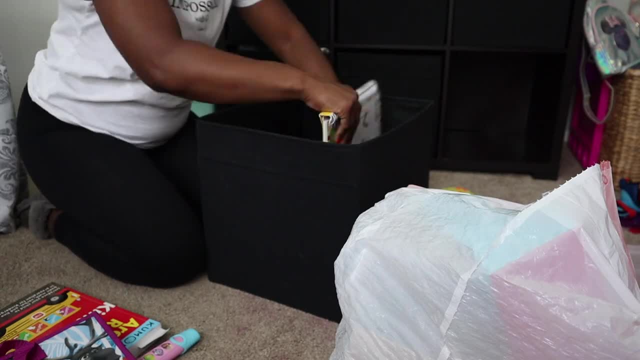 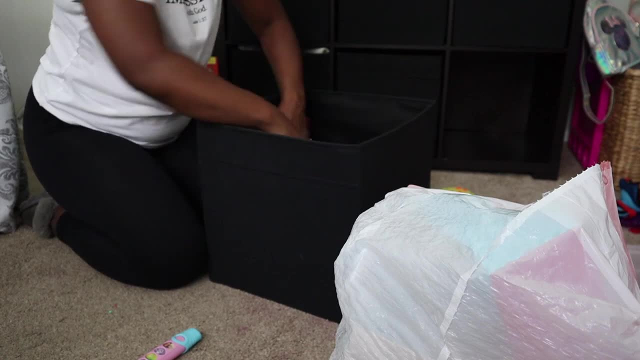 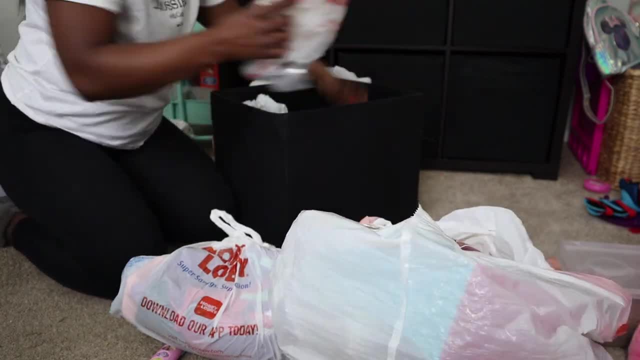 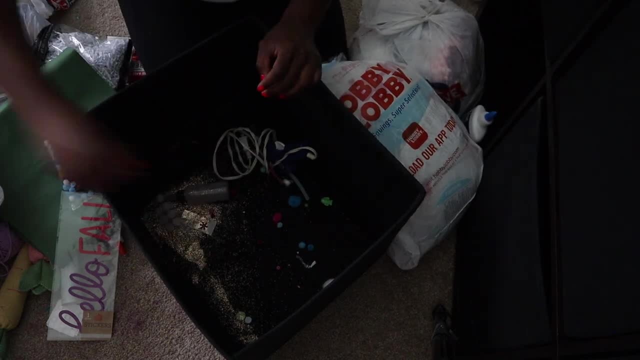 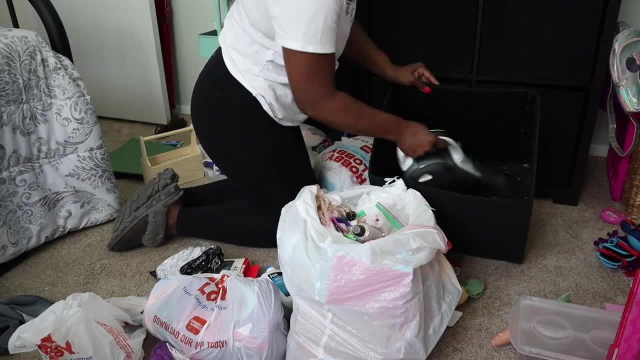 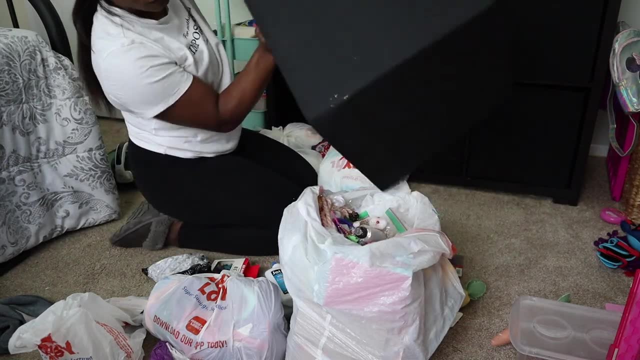 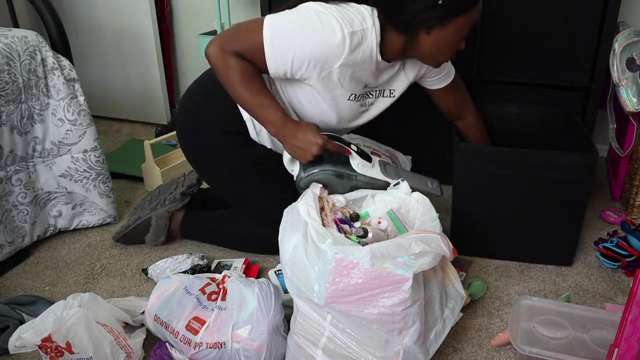 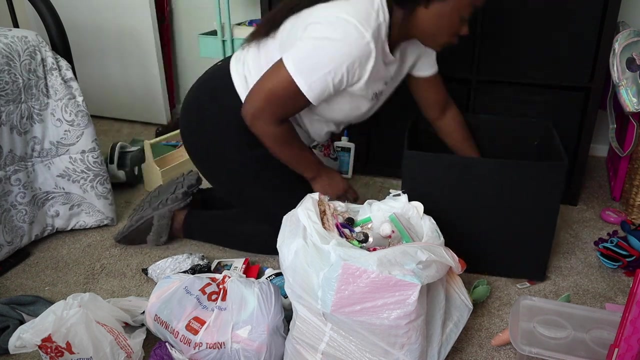 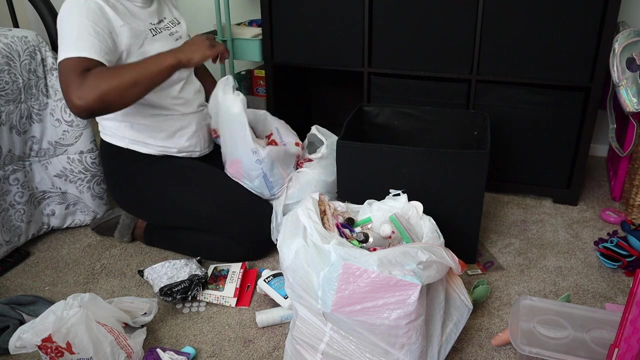 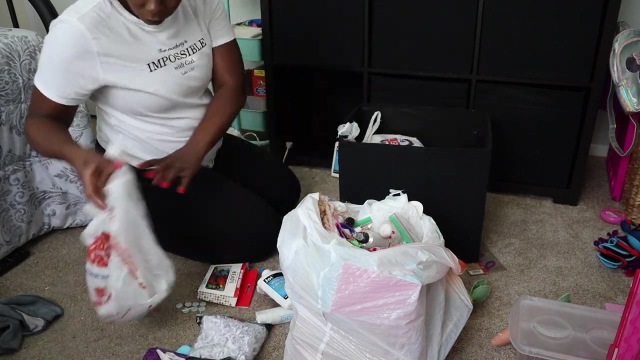 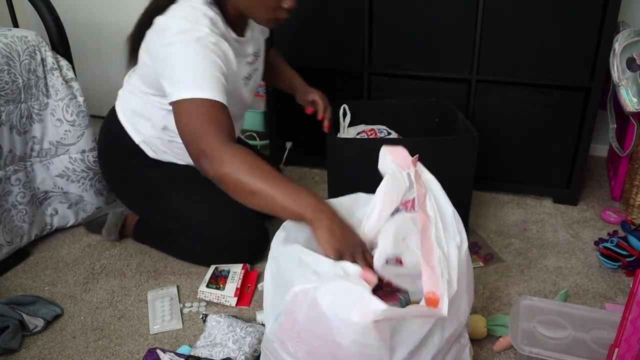 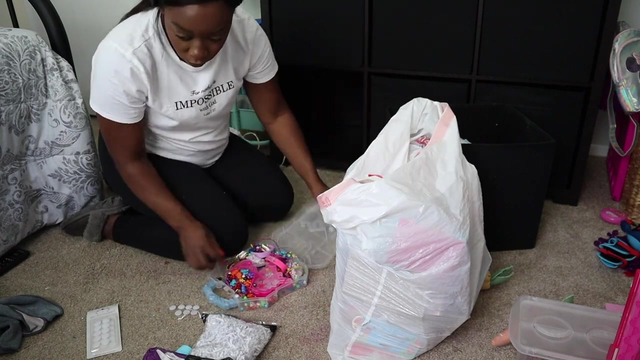 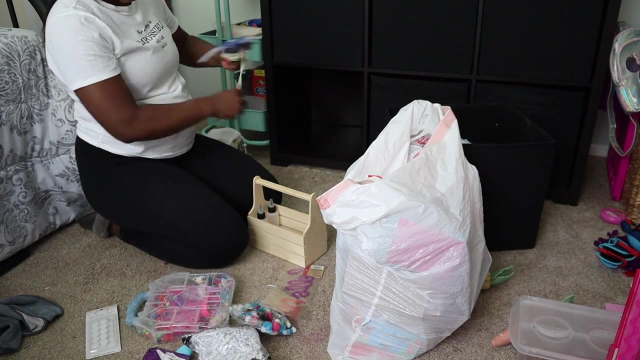 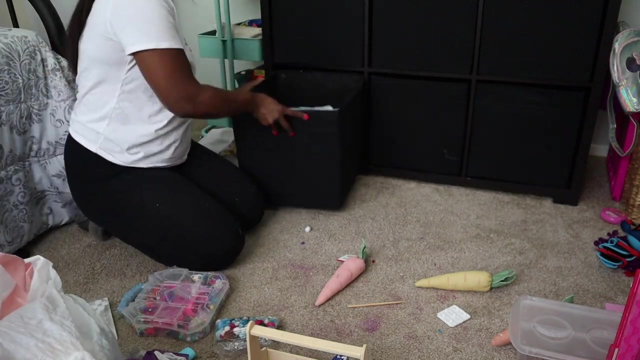 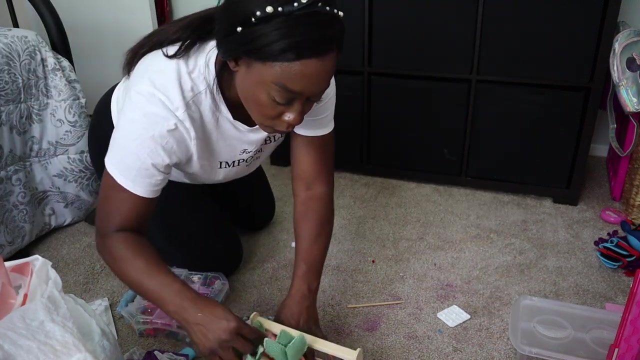 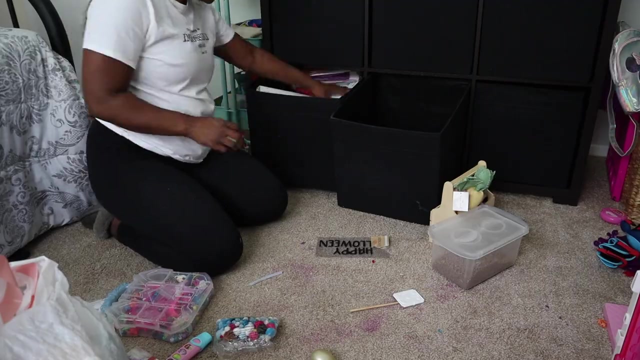 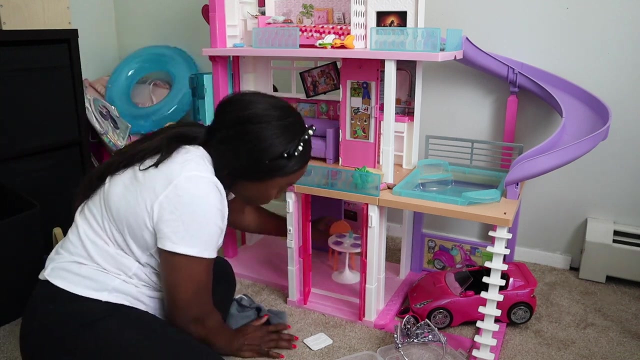 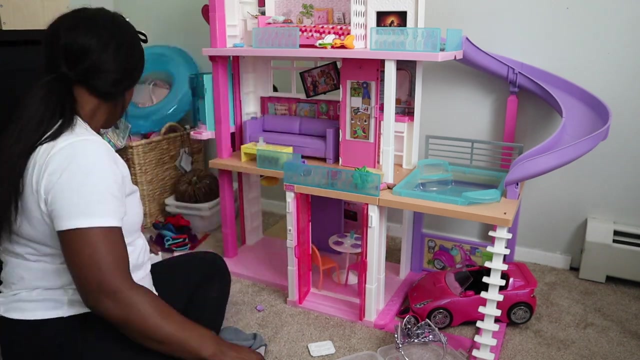 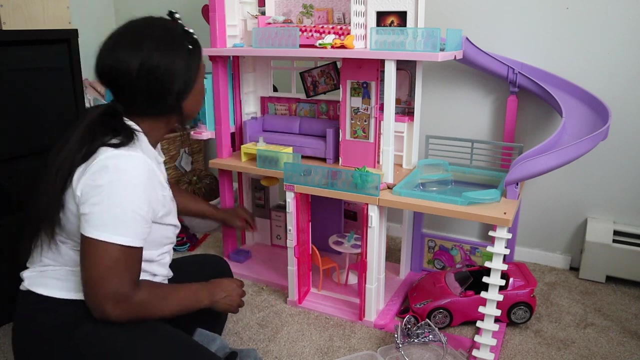 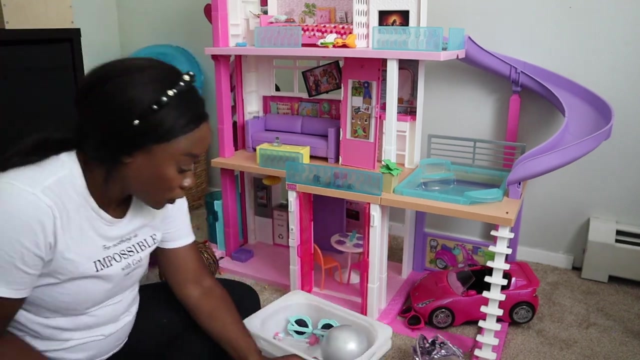 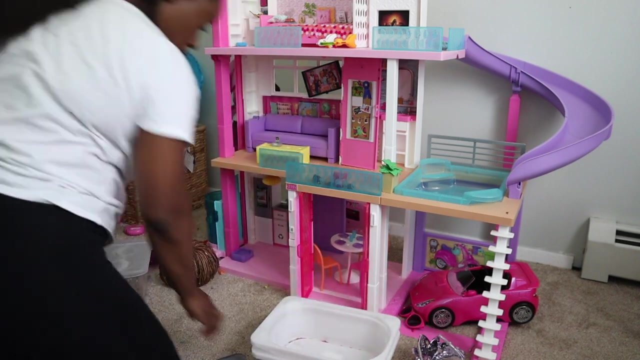 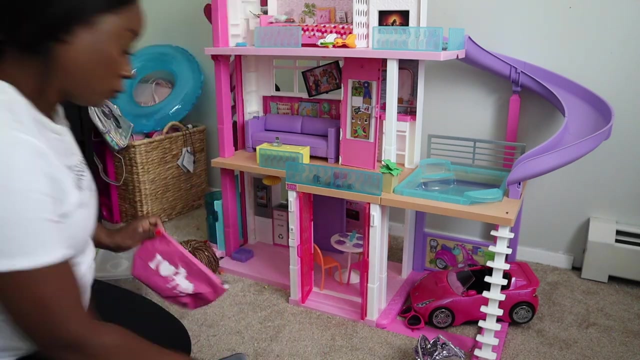 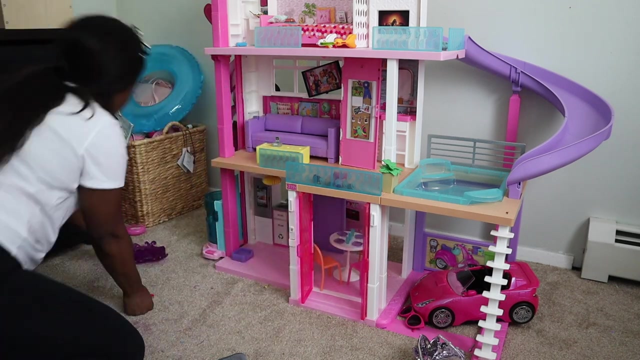 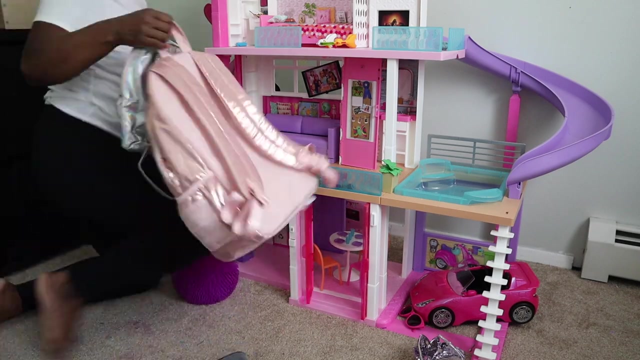 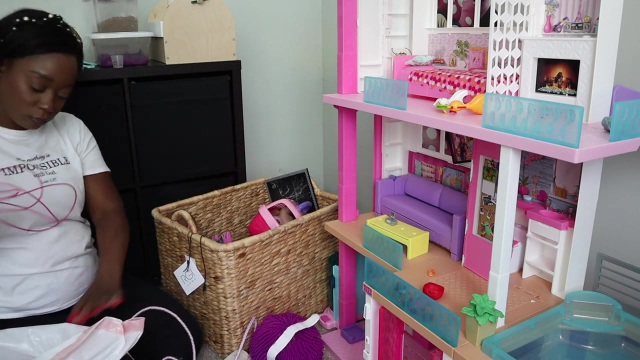 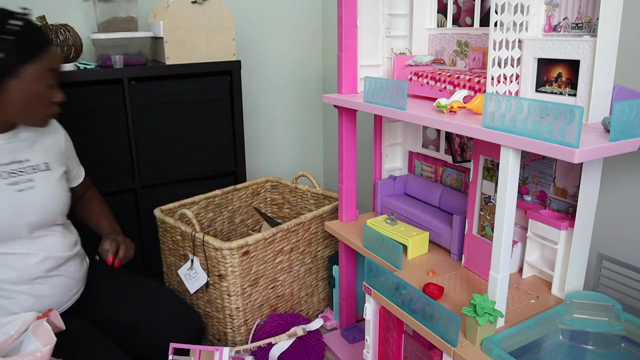 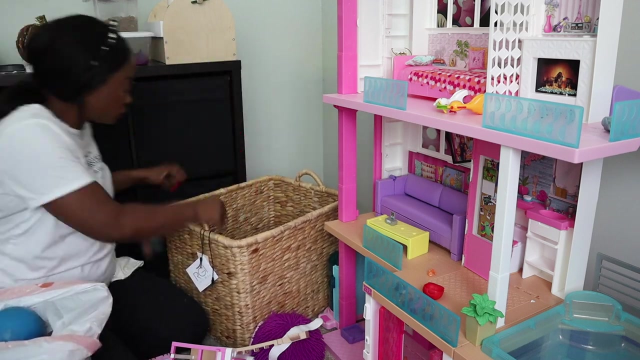 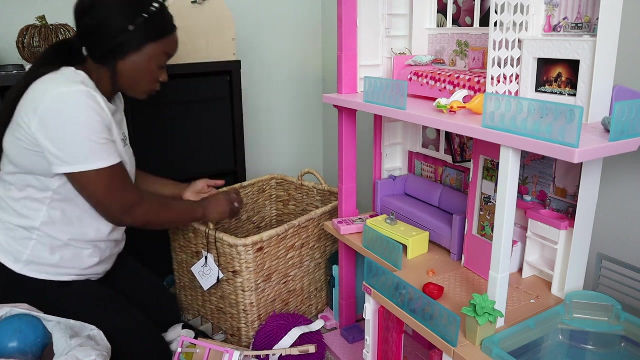 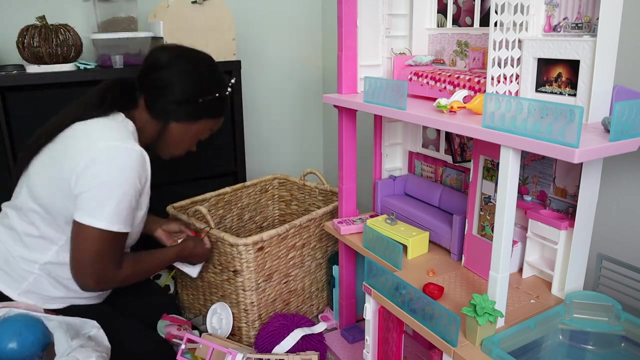 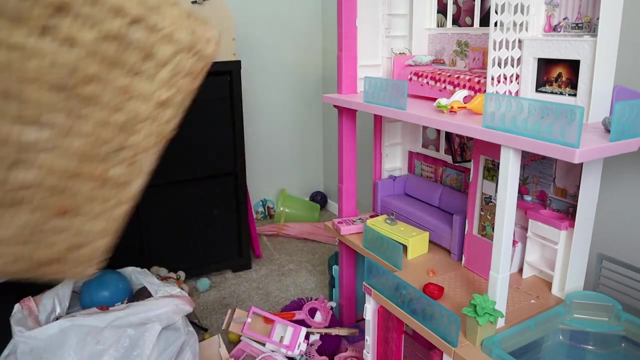 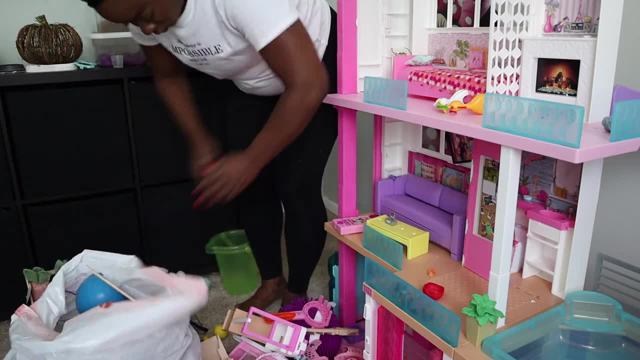 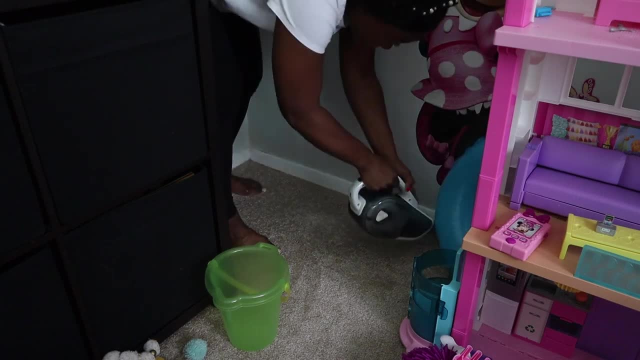 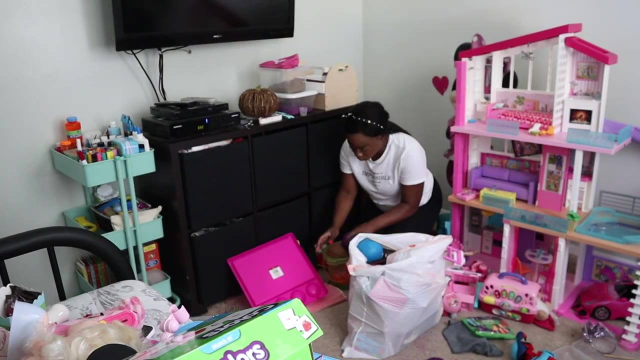 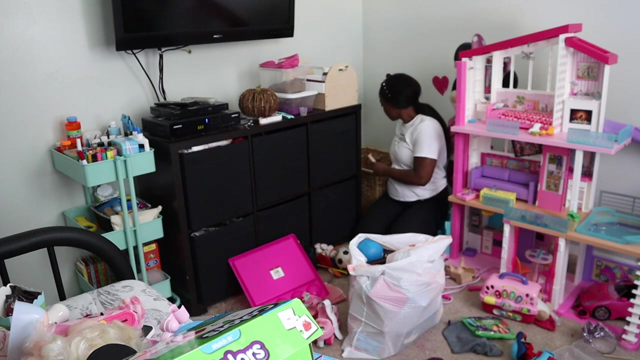 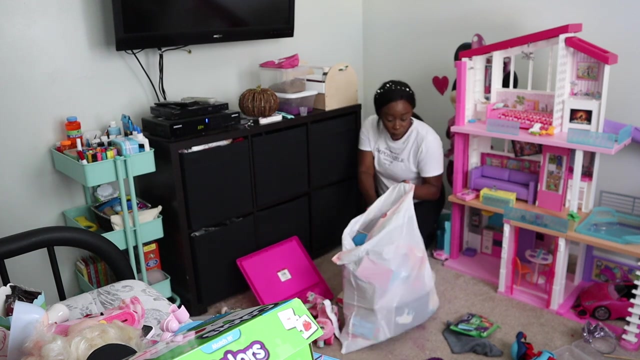 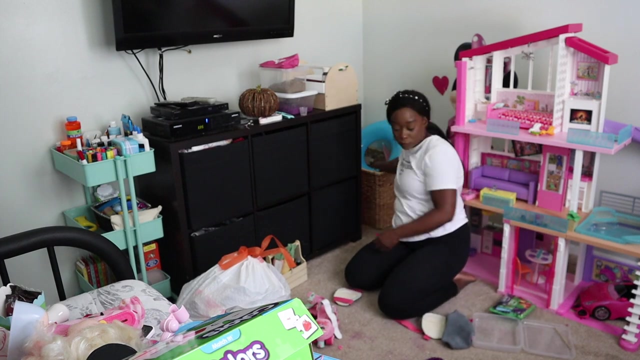 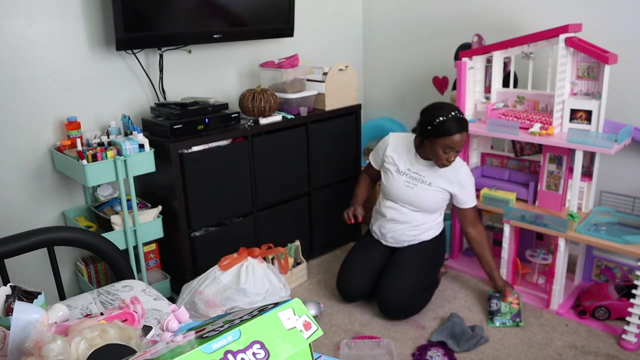 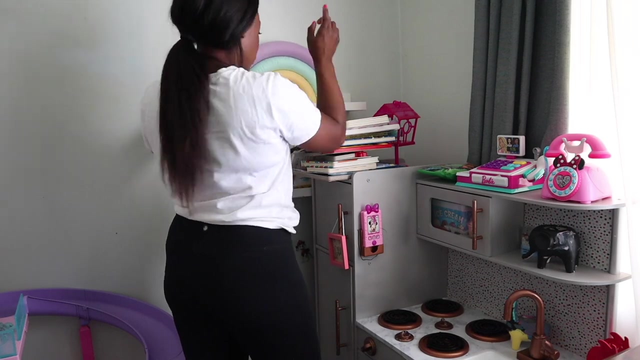 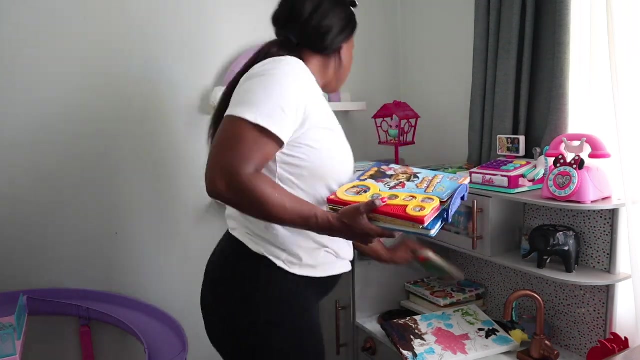 Thank you, Thank you. In this corner we had a bunch of random books, and some of them were books from when she was a baby, so I know I can actually store those away for any potential future babies. and then some of the books I actually wanted to bring upstairs so they could be something that we could read at night time. 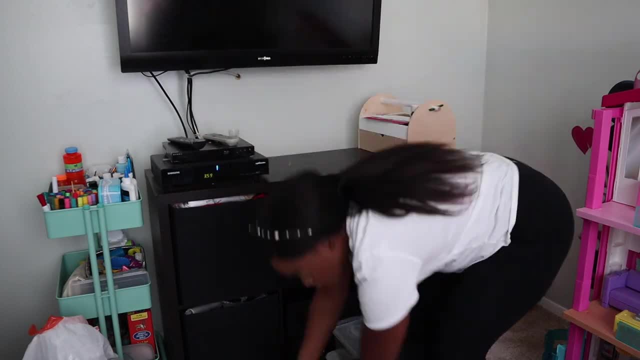 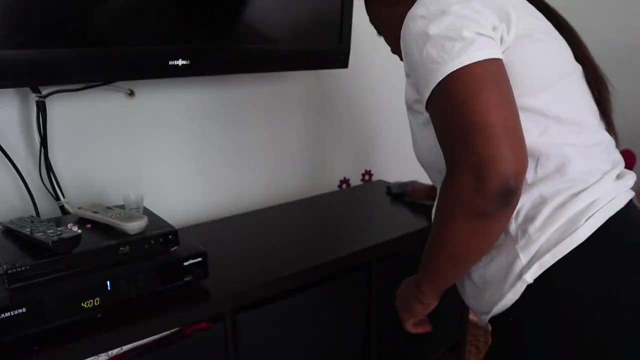 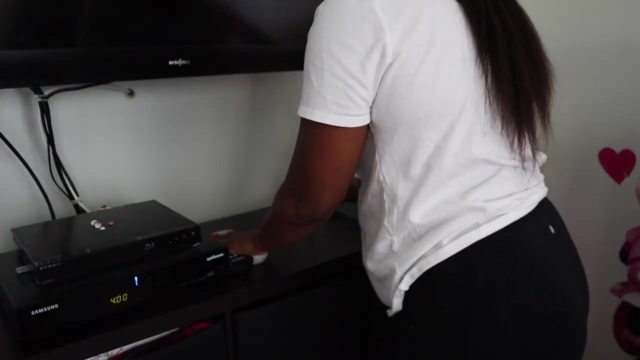 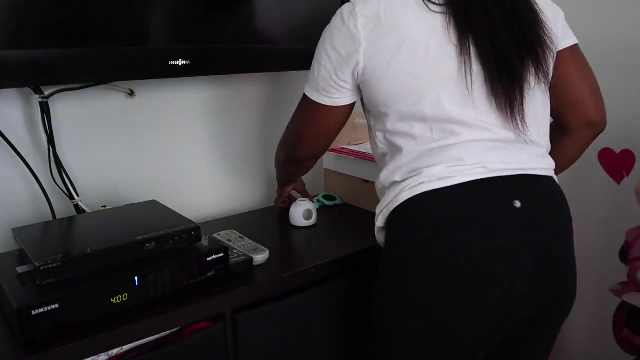 By bringing that cart down, it saved so much more room at the top of this furniture piece, so I definitely do like the less clutter-ness of it all. so I definitely thought that that was the best option for us right now, and what I ended up doing is just storing some of her like accessories, like her nails and her. 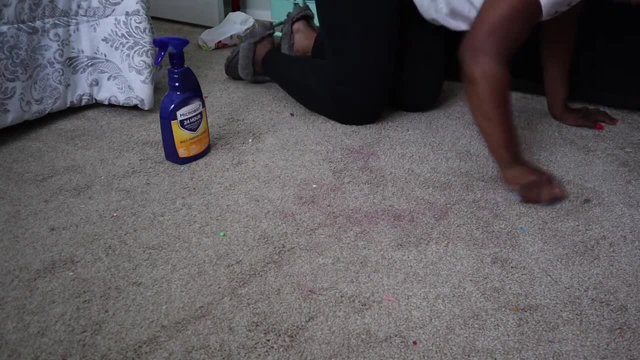 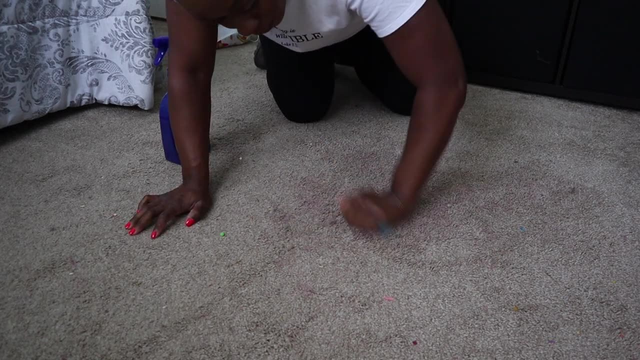 sunglasses and all of that stuff. I'm also going in with a micro band and a small little brush to try and get out some of the play sand that had fallen onto the floor. If you guys have been around for a long time, you know my struggle with this kinetic sand. 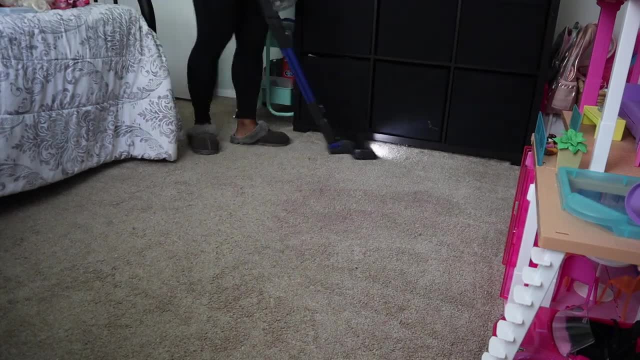 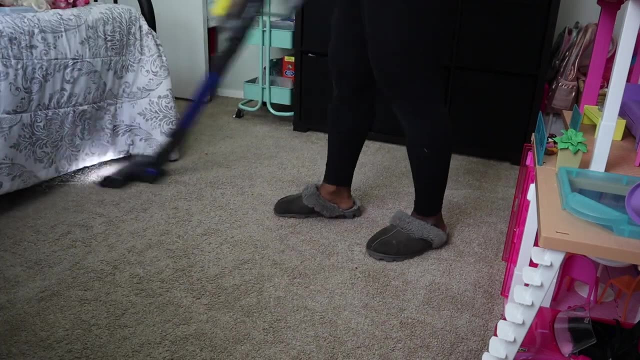 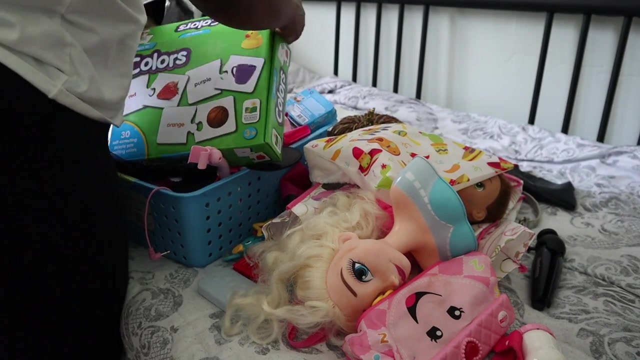 She loves it. so I don't want to throw it away. but I hate that it causes such a mess and really can get deep into the carpet. Just want to stay close. don't say a word. Ain't gonna leave ya, I don't wanna sabotage. 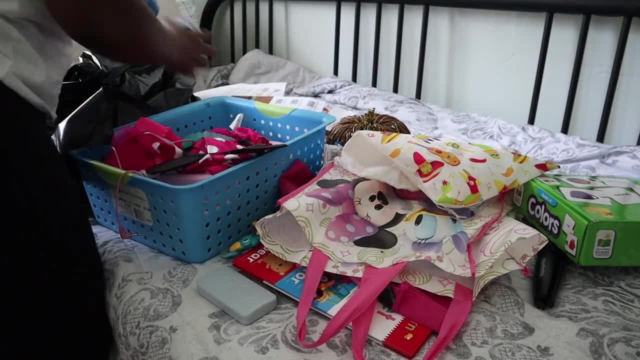 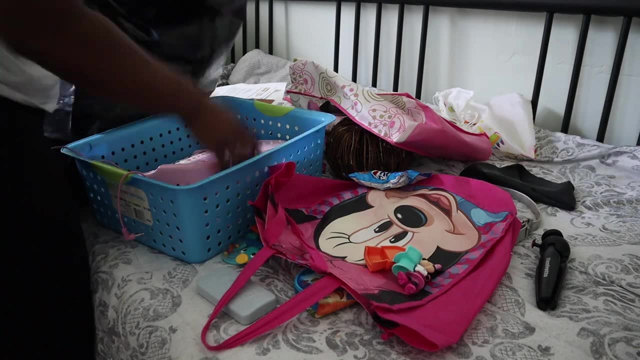 I don't wanna be the only one. I'm a successful person. I'm going to keep fighting With everything I've got, the work I've done, the hard work I've had to put in, the hard work I've put in.